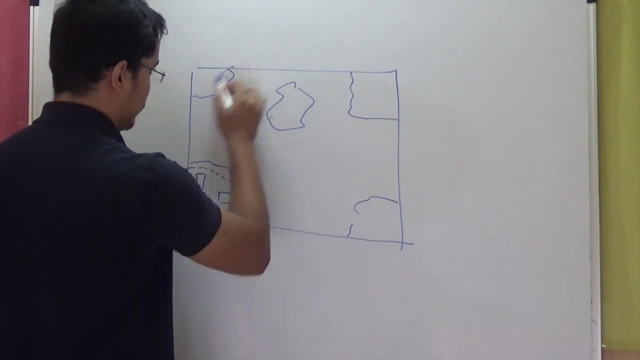 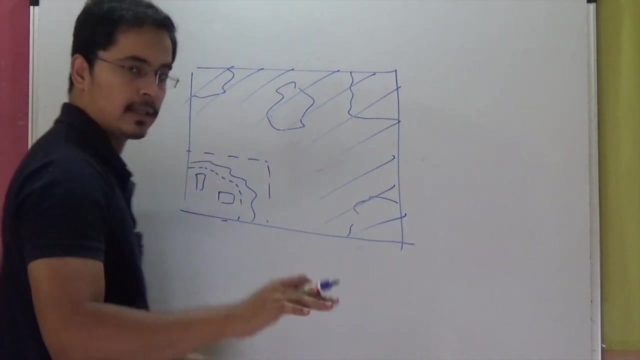 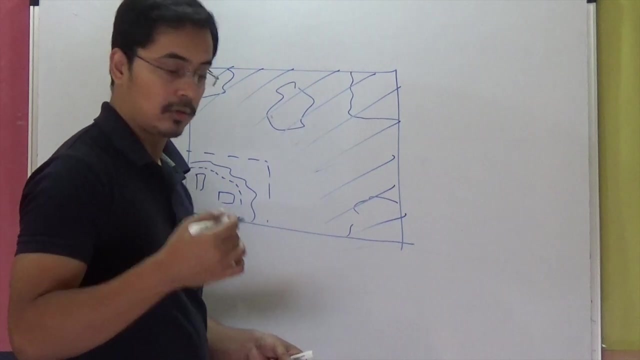 you don't see this area at all. this is all black. this is all black to you, right? you don't see this. you only get exposed to this area, right? so it is advisable, while you are building your infrastructure and army, to explore these other players and so that you know the most ideal routes for attacking them. 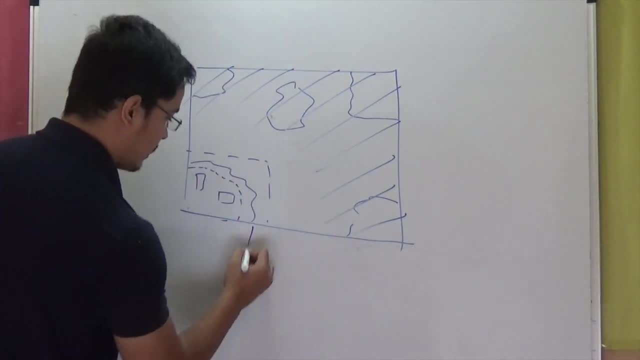 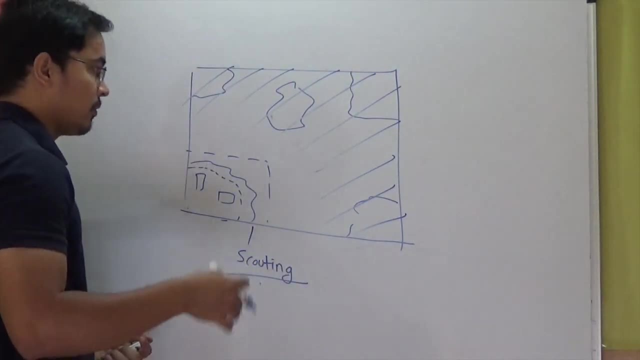 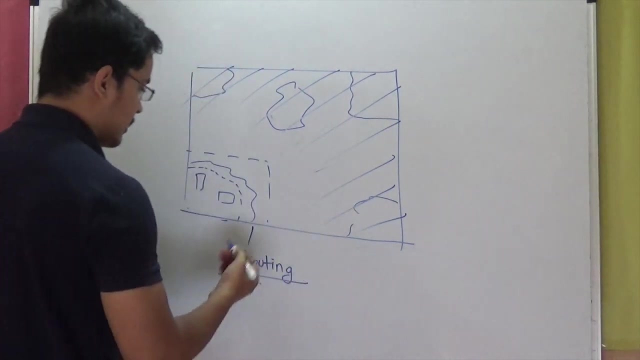 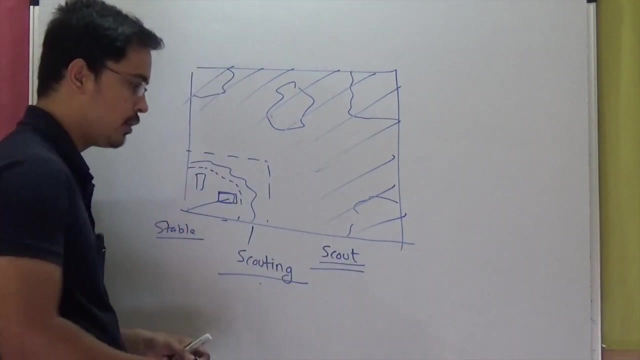 plan your strategy accordingly. right, so that is called as scouting. so you have to explore the area, you have to know your opponents- where are they situated, and their strengths and their weaknesses. right so now the scouting is usually done in age of empires, using a scout. so what is a scout? scout is a horse rider. basically, once you create your stable, you can. 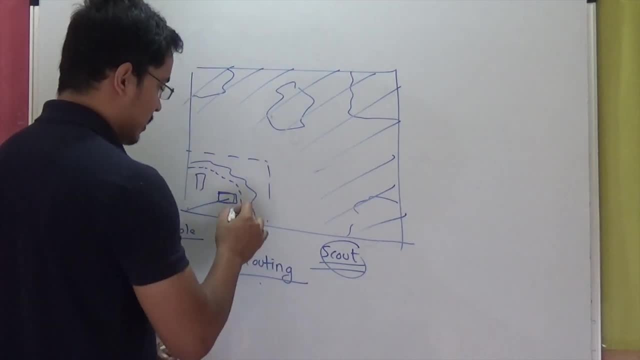 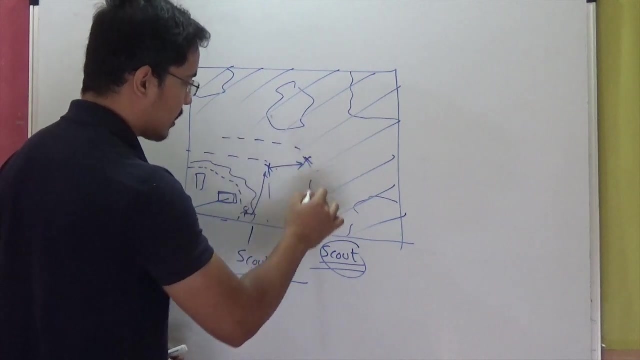 create a scout. once you create a scout, that scout is like this guy right on a horse: you can point it here, then he will ride here, then you can point it here, then he can ride it here. so as you keep on traveling your scout, more area becomes visible to you right, more and more area becomes visible to you. 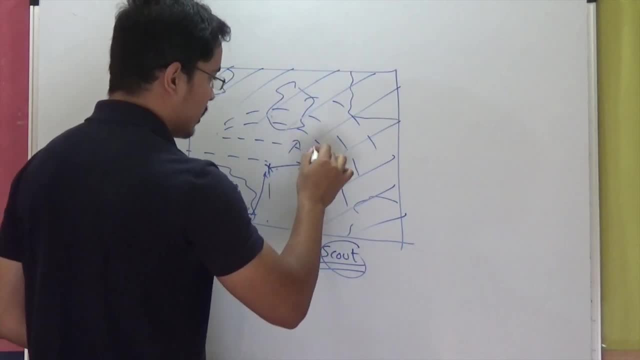 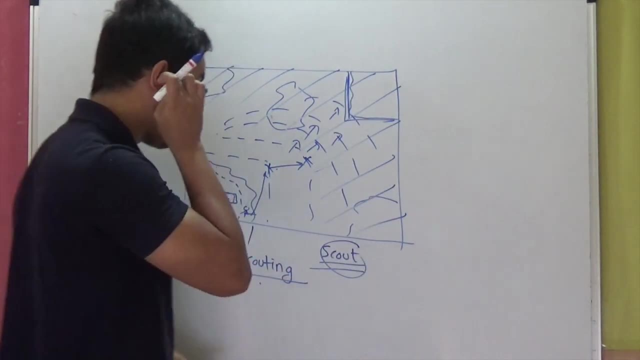 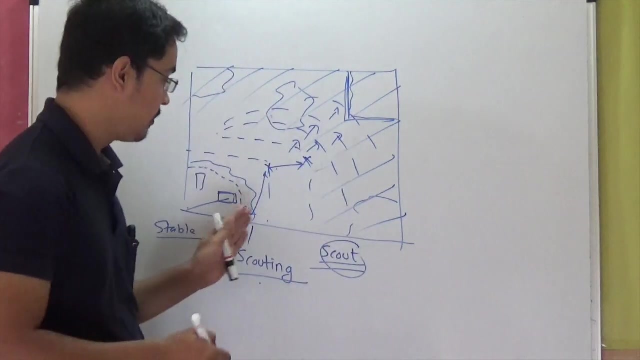 as your scout progresses, so You keep on pointing him forward, forward and forward until he actually reaches the city walls of the opponent, right. So that is traditionally how scouting is done in Age of Empires, right? And you have to keep that activity going on parallelly while you are building your infrastructure. 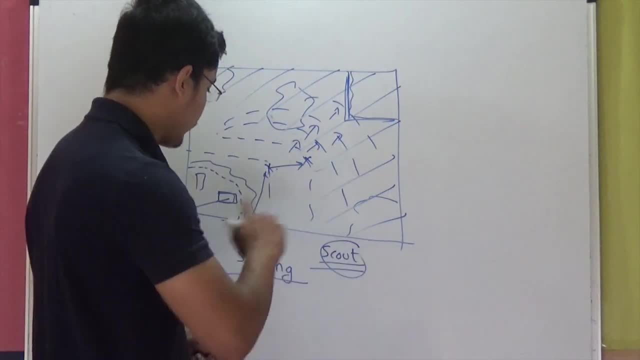 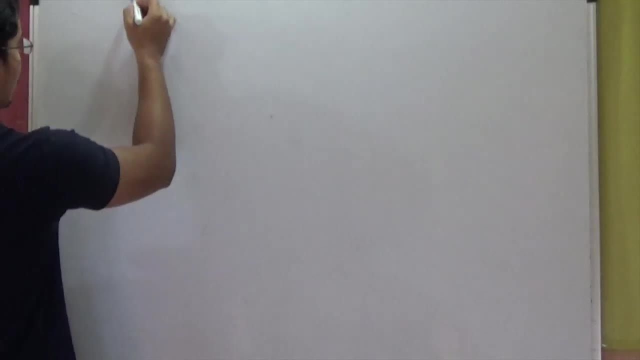 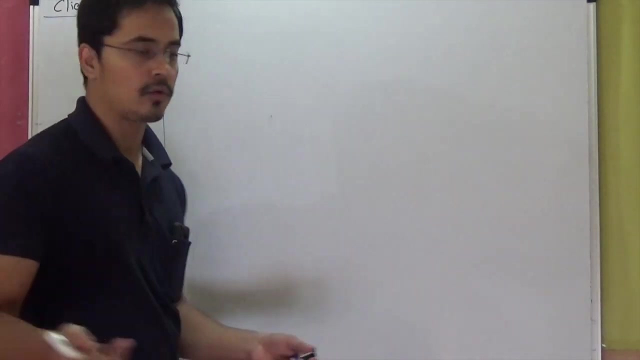 like you're generating your army or training them, or citizens, and gathering food and all those activities, right. So let's look at how this code will look like. Let's keep our client here, right. So client in this case is player. First thing we need to do is, in order to create a scout, is to have a stable. 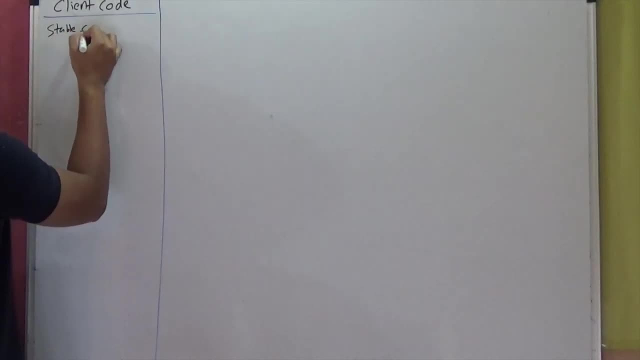 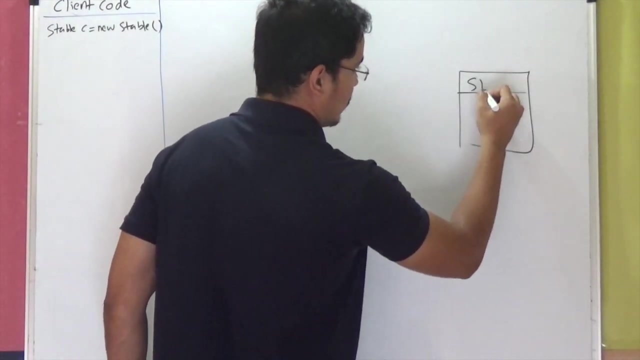 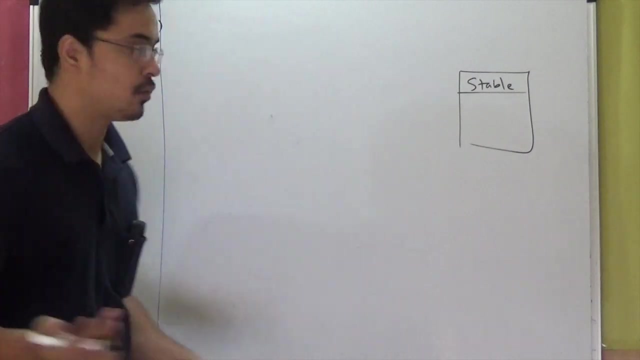 So you could say: stable C equal to new stable, And the entity involved here is stable right, Stable class. So you create a stable right. That is step one. So once you have a stable, now you can create a scout. 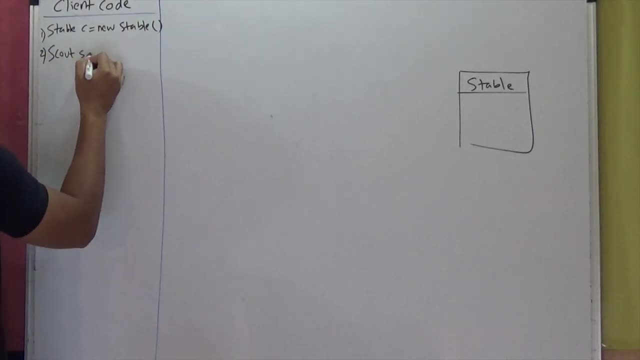 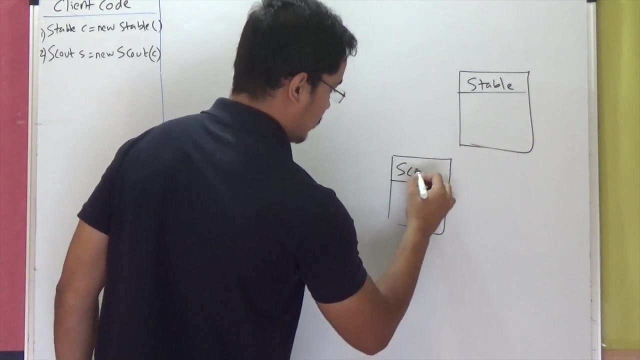 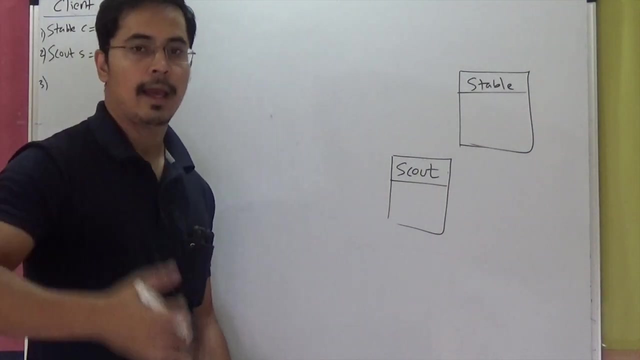 So you say: scout End S equal to new scout. So next thing you create is a scout. Once you create a scout, now you have to point him to some position where he has to ride in order to explore more area. So you have to say: sride, some method right? 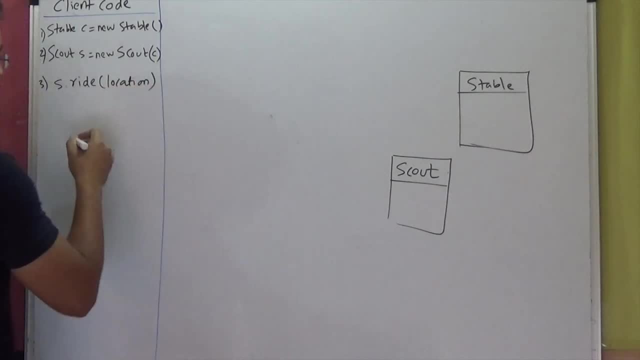 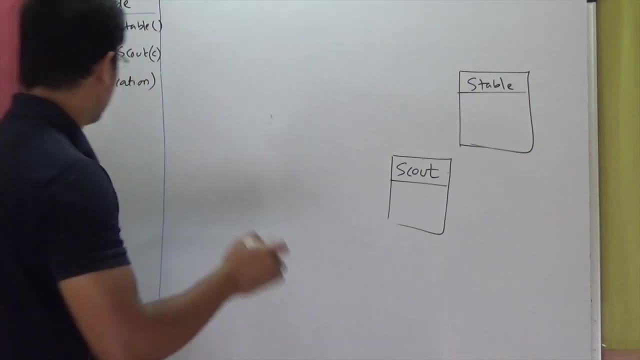 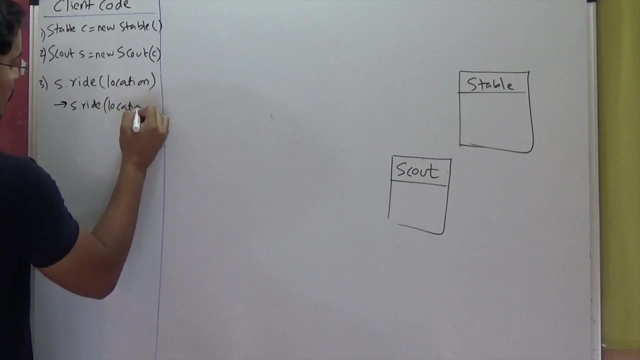 And you'll have to provide some location right. Once he does that, he reaches that location right, You get more Like, more area visible to you, So you can you have to again repeat this step and say, ride again to location two right. 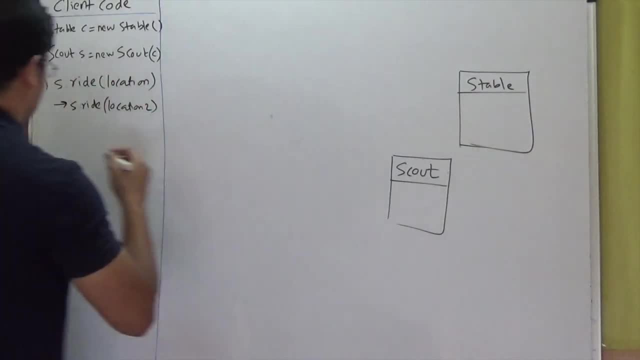 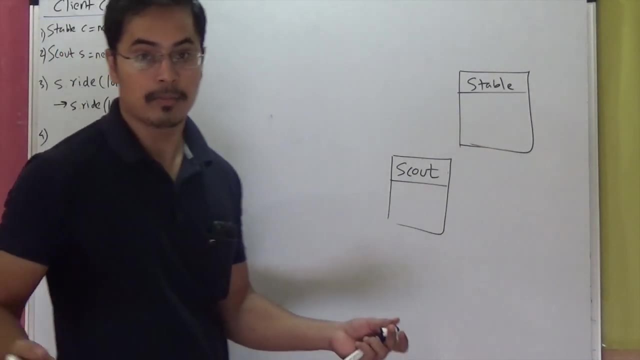 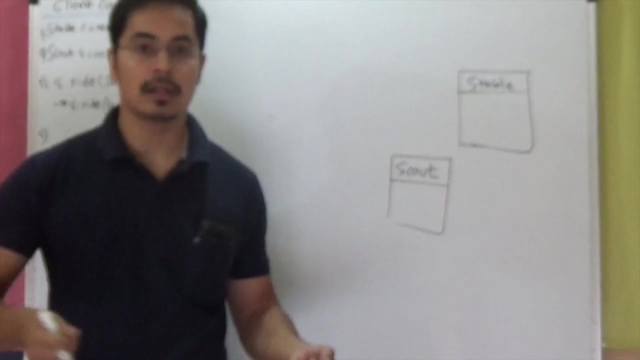 Again, keep on doing that: to explore more and more area. right Now, it's not that easy right, When you are entering an unknown territory, enemy area, there might be enemy soldiers who are guarding their area right, So your scout is unarmed. 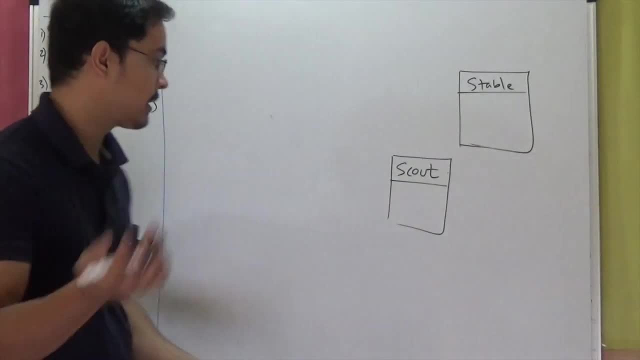 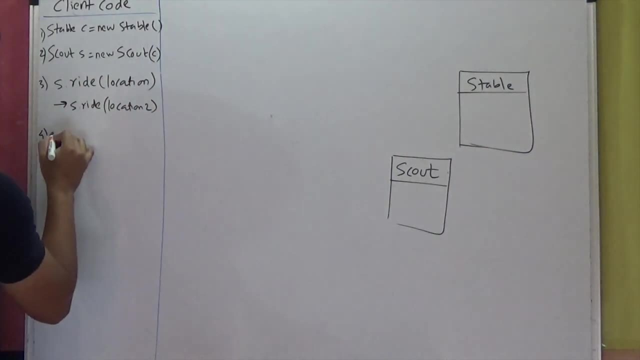 Scout is unarmed, So your scout may come under attack. So in that case it's advisable to create a paladin, a warrior riding a horse, a paladin. So let's say we'll create a paladin. Let's say paladin p equal to new paladin. 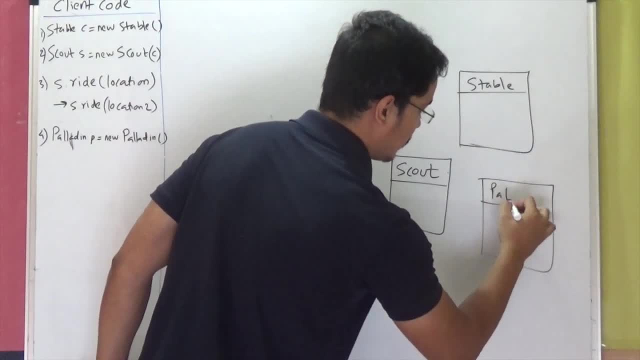 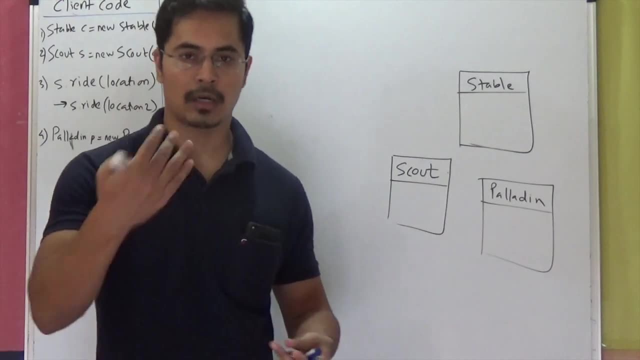 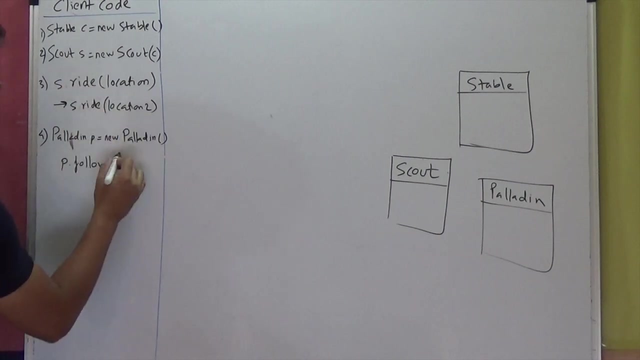 So we'll have one paladin. So paladin has to now follow the scout in order to be able to protect the scout in case the scout comes under attack, right? So let's say pfollow, it has to follow the scout. 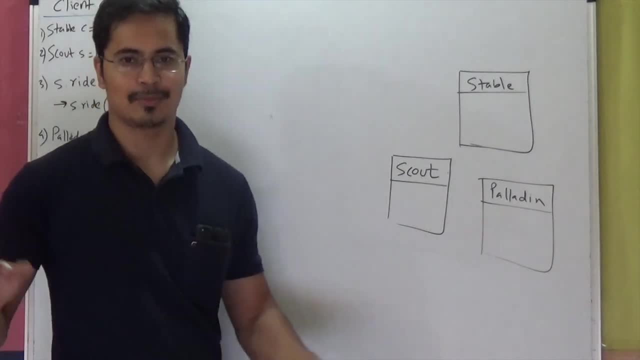 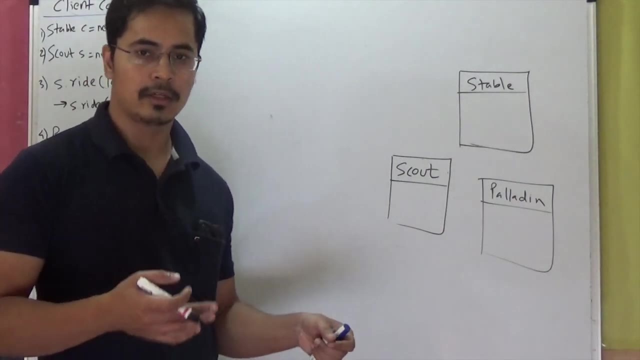 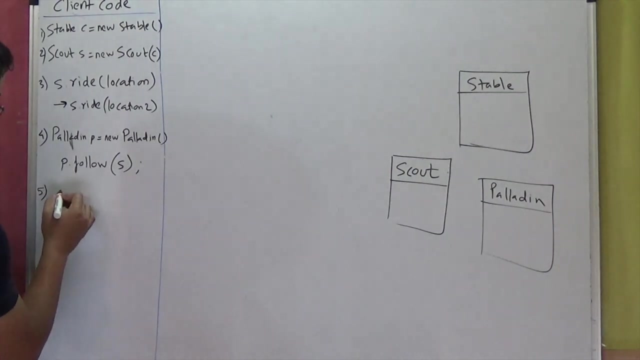 So scout object like Brienne is protecting Arya and Sansa, right, In case you reach a point where your paladins and scouts reach that enemy territory- now, enemy territory is visible, right, You want them back. So you will have to write something like: okay, scoutreturn, right, 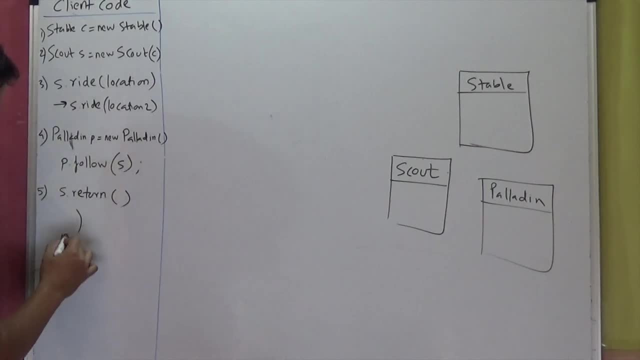 And scoutreturn. so paladin is following, so paladin will also return right. So this is all you need to do, right? A player has to do these activities manually. So basically, when player is doing all this using the interface. 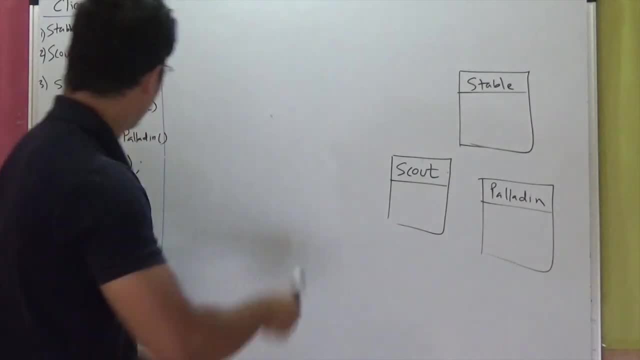 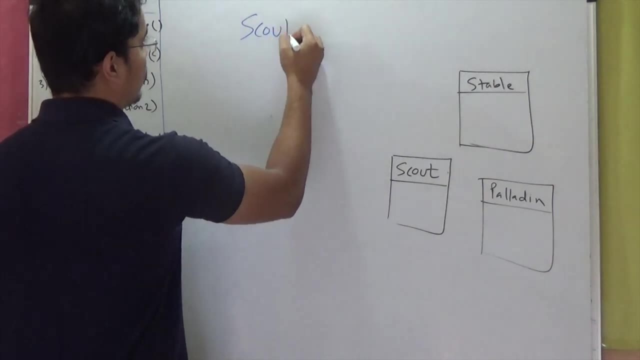 clicking the mouse and generating the objects. the behind the scene code is pretty much like this: right? So this is all being done to carry out a task of scouting, right? So scouting is the task, and in order to carry out this task, 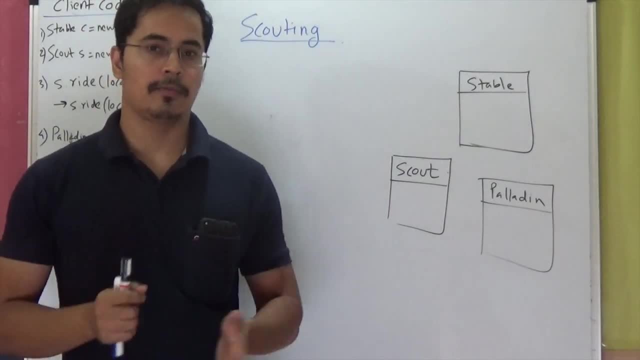 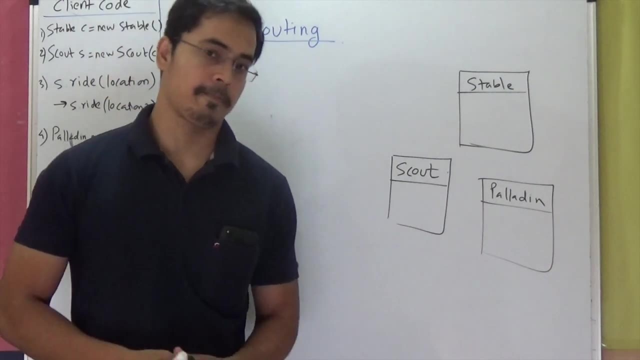 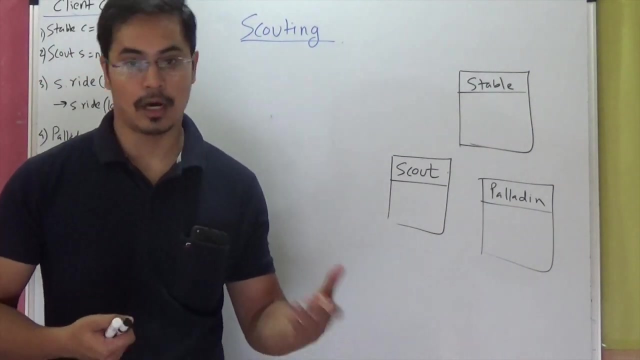 we are creating all these objects and writing all this code. It doesn't stop here. This was the most optimistic case. right Now there are complications. For example, your scout can get killed, right? Yes, paladin is trying to save the scout. 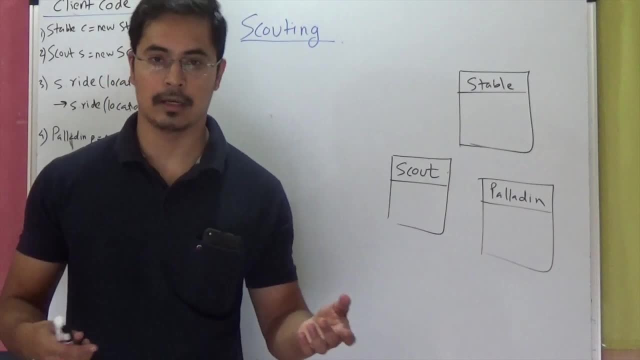 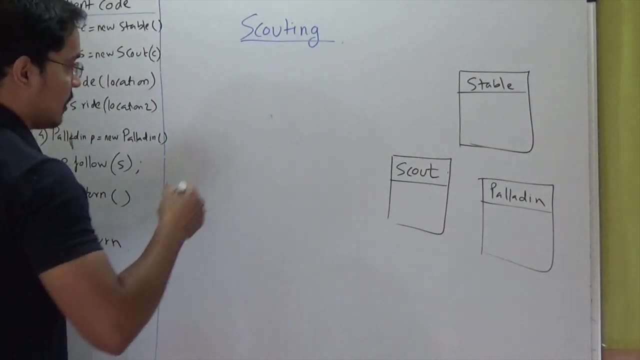 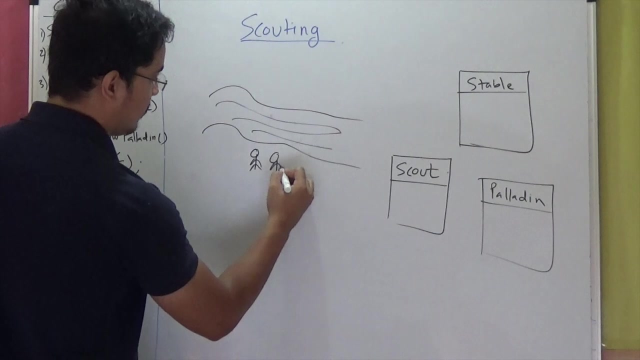 but both can get killed under heavy attack from the enemy right. So that is one problem. Second problem: the scout and paladin might come into a point of area where there is a river right. So there is a river. here are your scout and paladin. 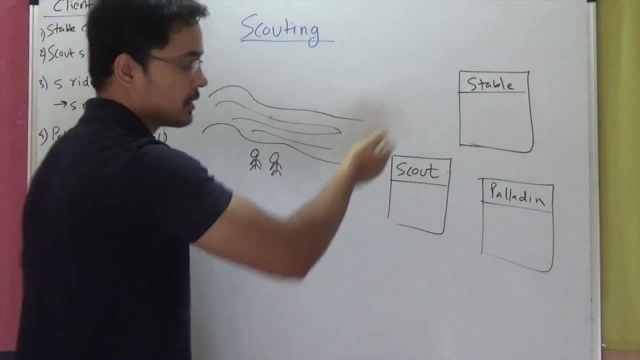 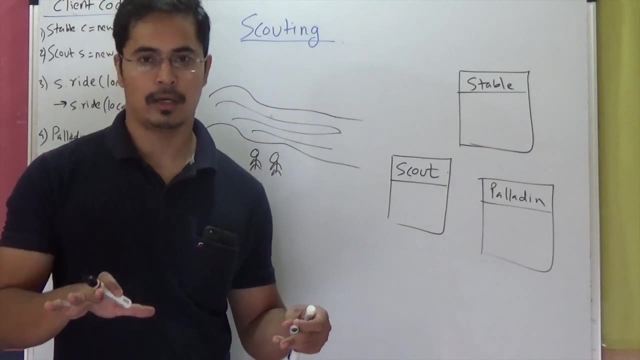 Now in order to explore further, they have to cross the river, but they are both on horses and they can't cross the river. So your scouting mission is now halfway through right, And in the meantime, you have to also pay attention to your own city infrastructure and everything. 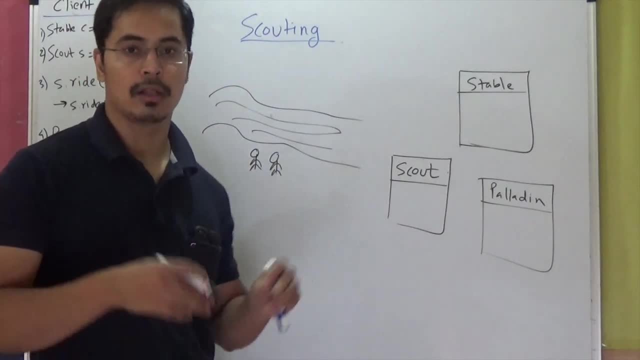 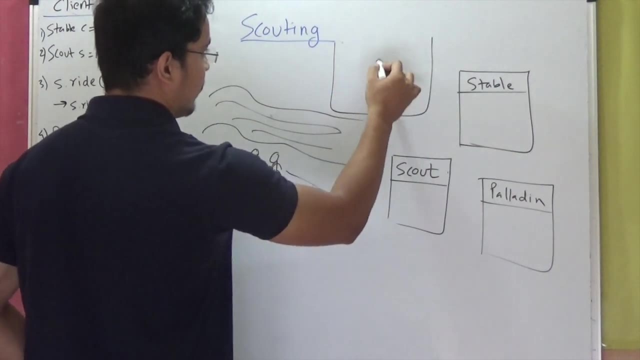 So you have to pay attention to your own city infrastructure and everything. So you don't even know at times that your scout and paladin are stuck there, right? So that is one more problem. And you somehow reach the enemy territory. So this is enemy territory, right? 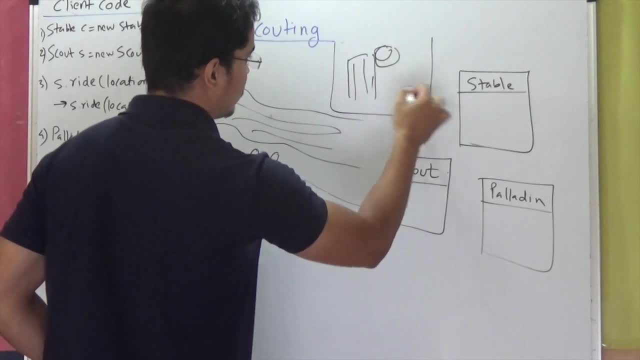 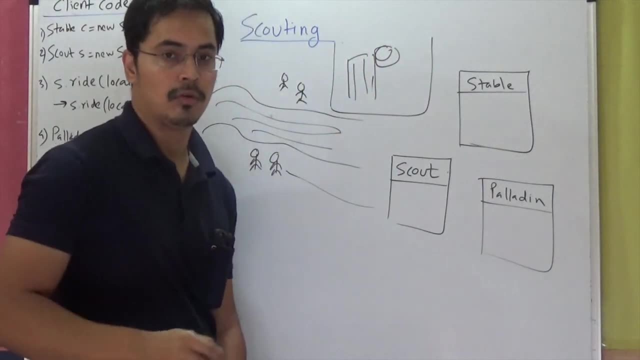 So you see these enemy buildings, enemy castles and everything. Now the problem is, your scout reaches here and paladin right, So there are walls now. So you can only partially see the enemy territory. You want to explore it to fullest right. 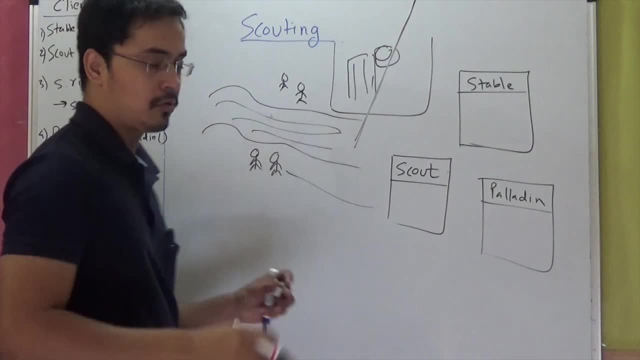 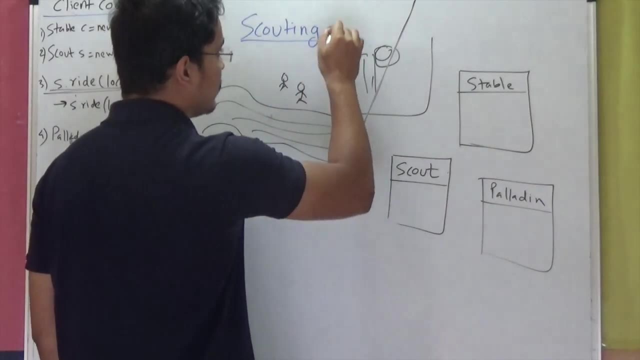 So, again, you have to start new activity off, You have to, as I said, this step scoutride, you have to keep pointing him to this position, this, and hope that there's a, there's a breach in the security. 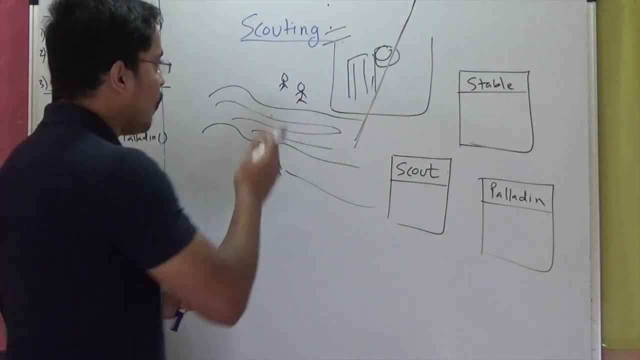 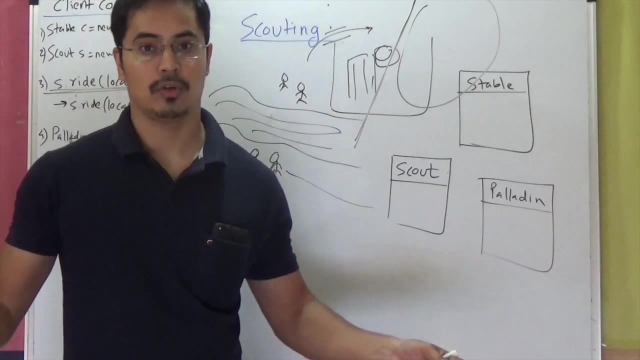 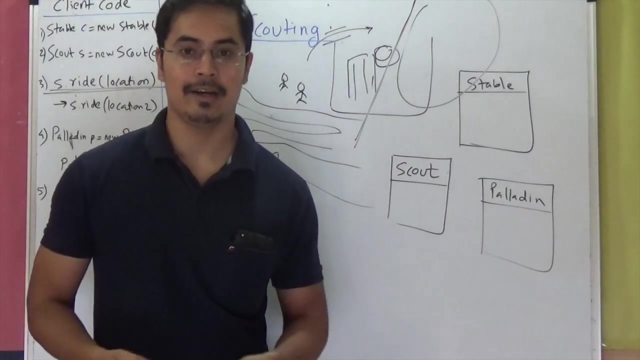 or there's a gap in the walls of the enemy territory And hopefully your scout can sneak into that gap and explore the enemy territory in full right. That is one more issue. So lots of issues. lots of manual actions have to be taken by the player, the user right. 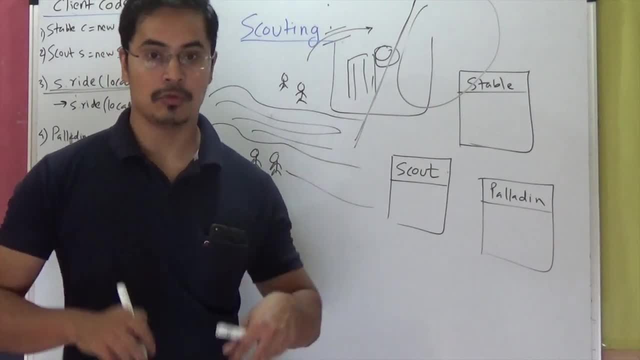 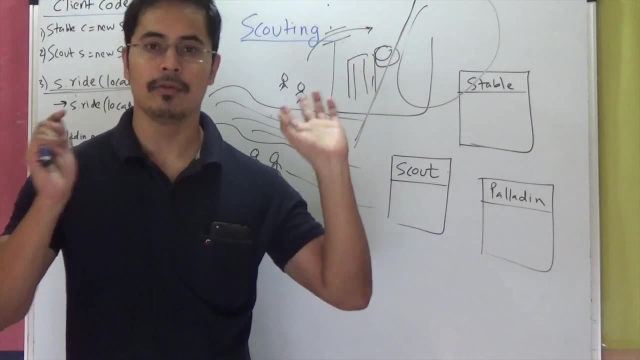 And meanwhile, as you are doing all this activity, you, as a player, might come under attack from other enemies, right? So you might lose track of these scouting activities and they might get killed eventually. So it's a pretty tedious task, I would say right. 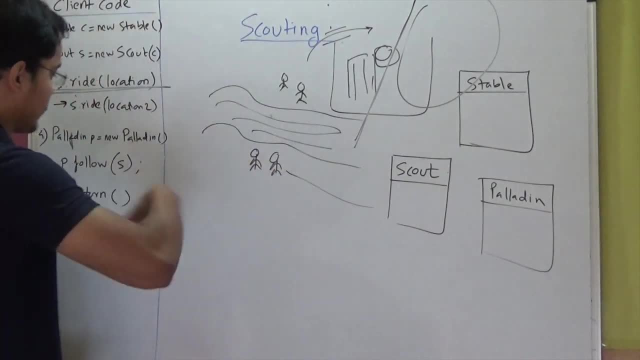 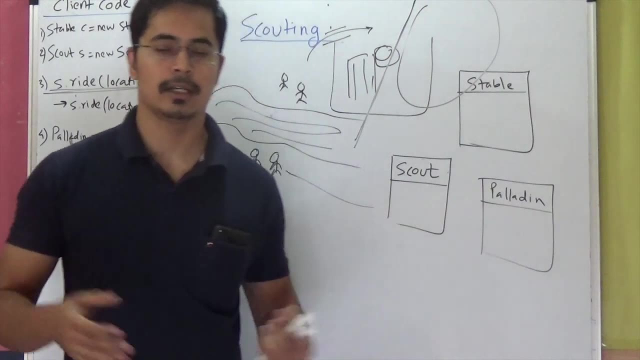 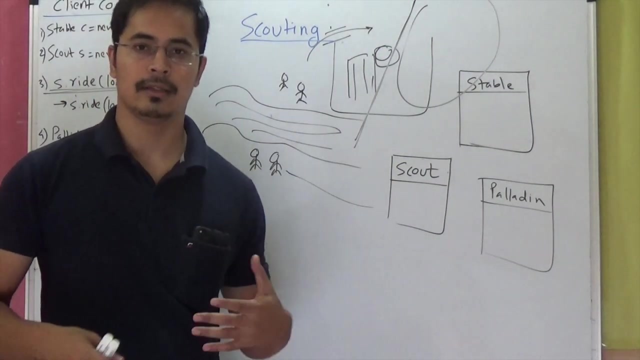 Now, what if this complex system of scouting, can we simplify it? I'm a developer, I'm a designer, a program designer, and we have object oriented programming at our disposal. So can we, Can we simplify these things for our users, for our players? 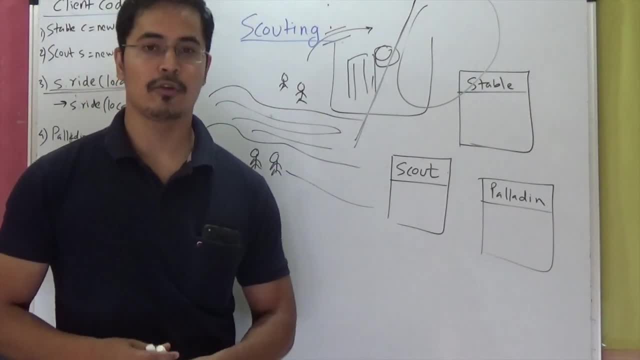 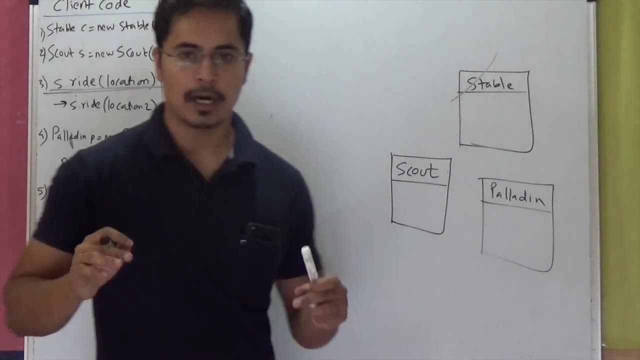 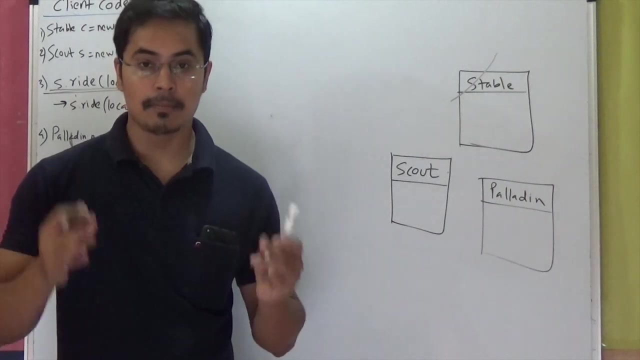 Yes, certainly we can, And for that we are going to use facade pattern. So this code now will make it simpler for client. So facade pattern is used in order to create a higher level simplified interface in order to access a complex subsystem, right. 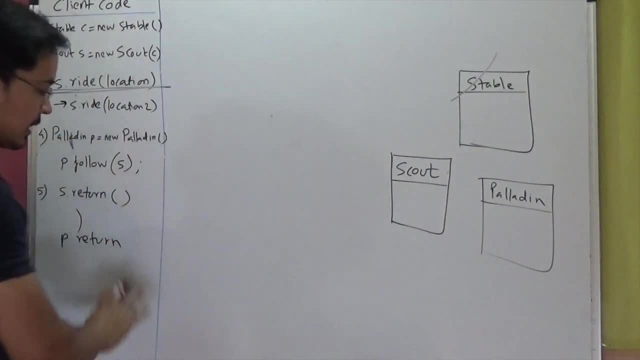 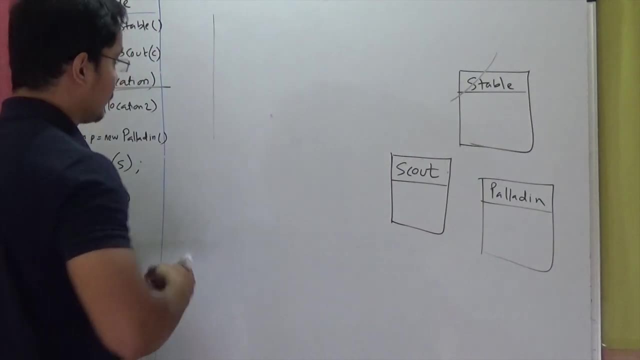 So I'll explain that, don't worry. So instead of writing this code, I'll explain this code. So, instead of writing this code, I'll explain this code. So, instead of writing this code, I'll explain this code. What I'm going to provide to my users are: I'm going to create an entity to class called 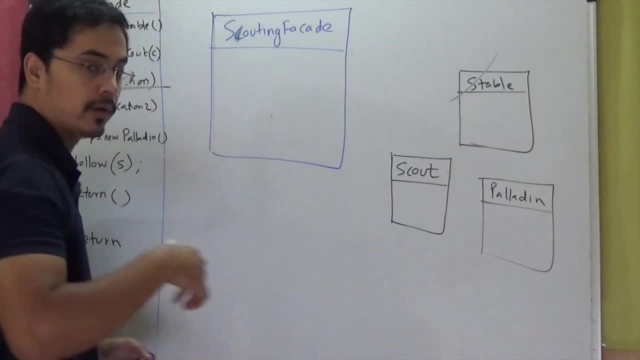 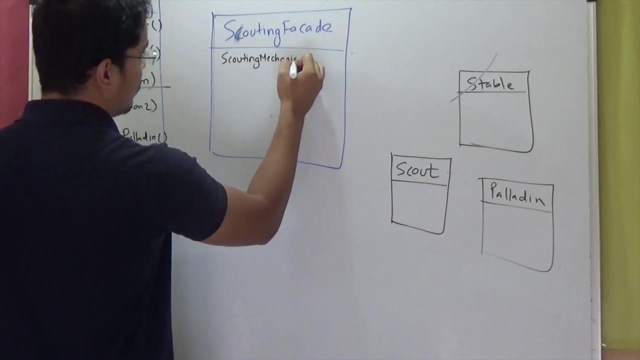 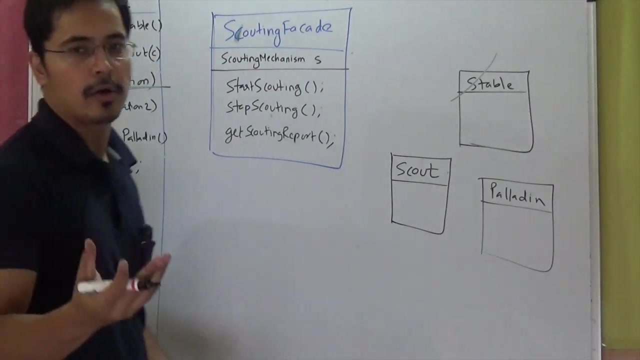 as scouting facade and I'm going to go one step ahead and create a composition here: Scouting mechanism. I'm going to compose an object right And this scouting facade will have methods like: start scouting, stop scouting, get scouting, get scouting, report. it's like a remote control, it's like i'm giving you access to a functionality. 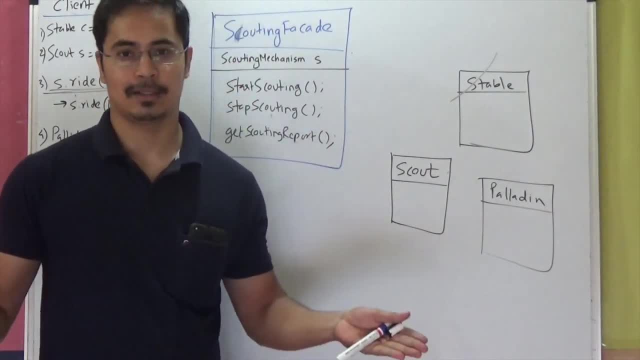 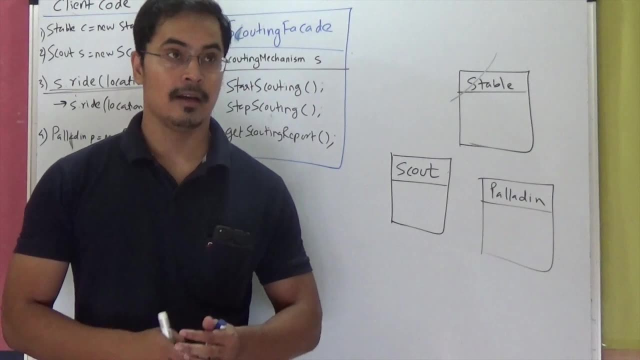 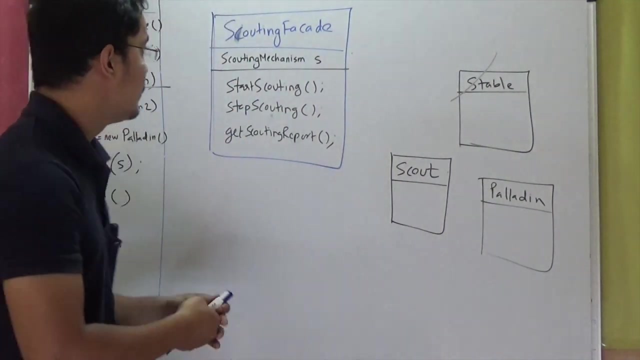 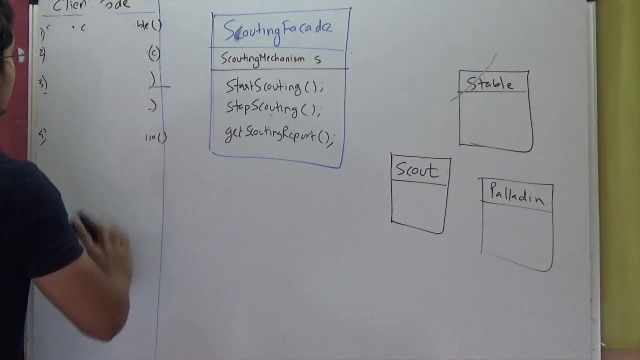 a complex functionality through a simpler interface. you remember the video where we are discussing object-oriented programming concepts and i was explaining the air conditioner example of air conditioner and the remote, why it is given to you. so it's very similar to that, right. so this is my facade class right, and the client code right is going to be now much, much. 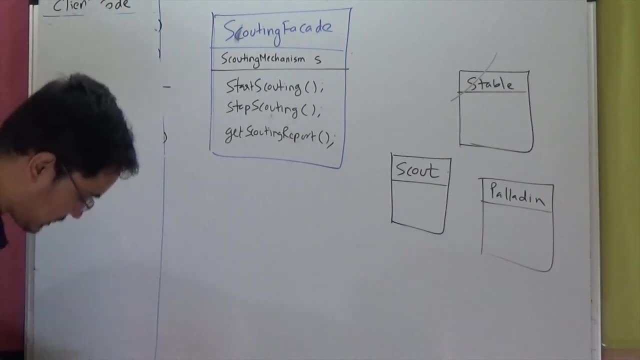 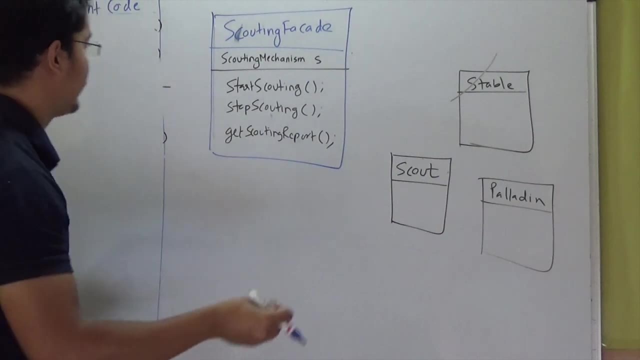 simpler, so the client code will not be this much complex and we'll say so: this is my client code. code will be dependent on the actions taken by the player, the user, end user. so i'll say i'll just create a scouting facade so he will click on the. so there will be a toolbar. 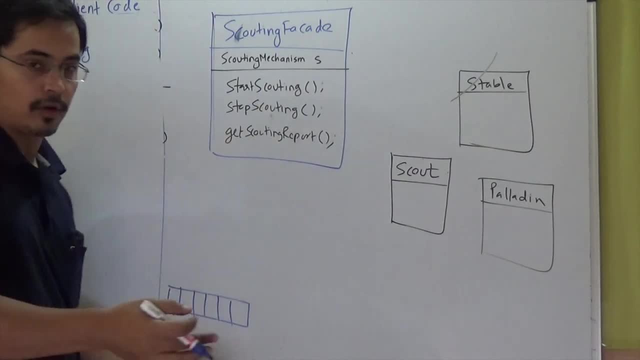 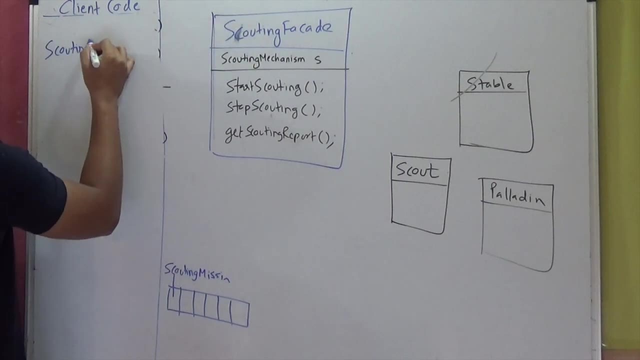 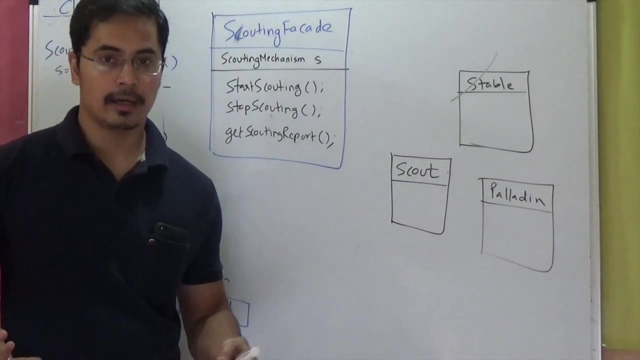 right on the bottom of the screen for user and he just had to say scouting mission here to select the scouting mission. it will create a scouting facade object s equal to new scouting facade, now based on the era in which the user is playing. there are eras in the game of 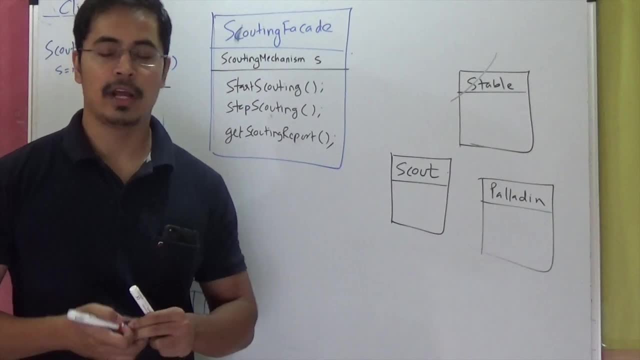 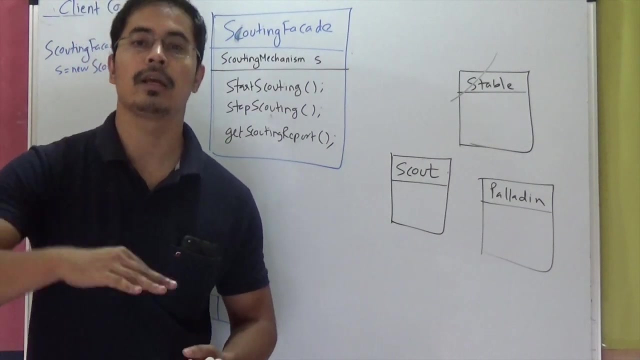 in the age of empires. so you have medieval age, you have modern age, you have ancient age And once you generate sufficient resources like food, silver and gold, you can choose to transform yourself from one era to another. right, If you have played that game, you know this. 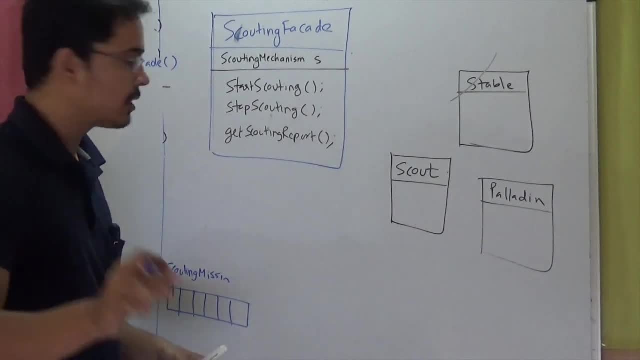 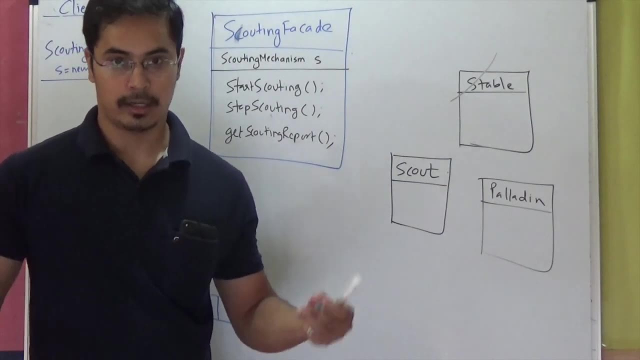 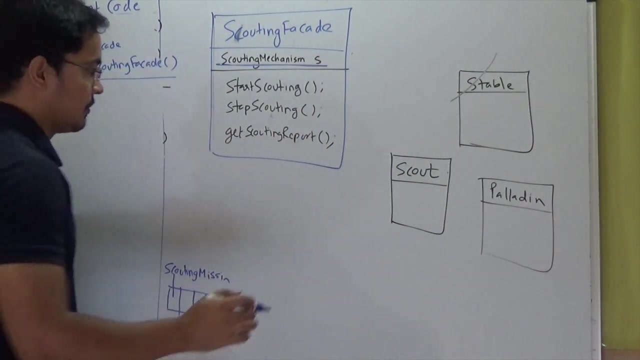 So there are different eras, right? So why I am talking about them? So once you create this scouting facade object in your client code, according to the era that you are in, the player is in the scouting facade will generate a concrete implementation for this composed scouting mechanism. 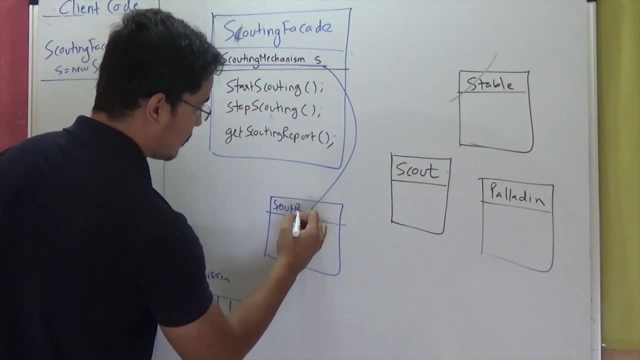 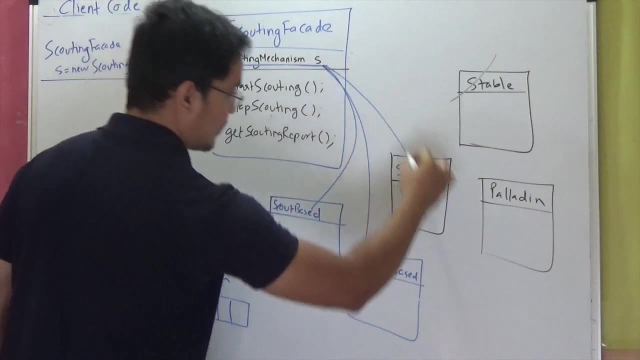 So scouting mechanisms could be scout-based. right, It could be. if you are in modern era, then it could be drone-based. Yeah, it could be motor-based, like you have vehicles, not so modern, but Newton era, right. 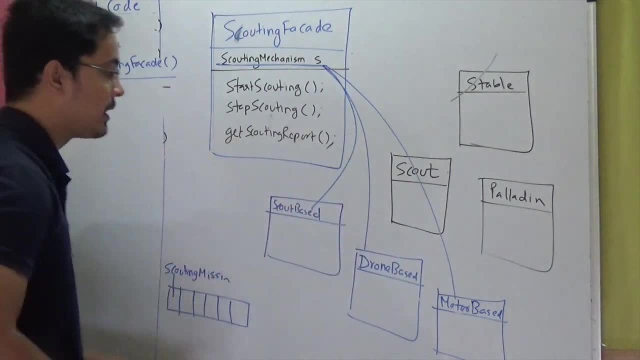 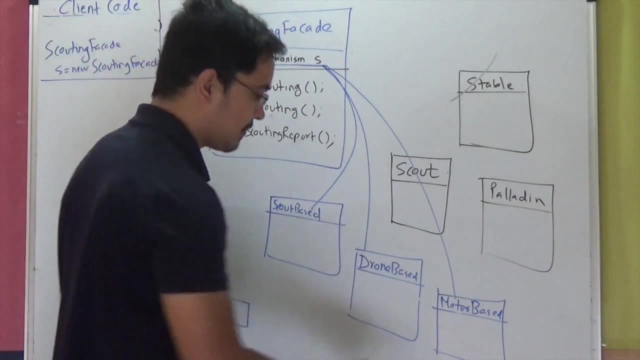 So motor-based scouting. So there are different concrete implementations of scouting mechanisms: Scouting Scout-based, that is, horse-based, Drone-based- the ultra-modern era- And motor-based, using a car or tank or something like that right. 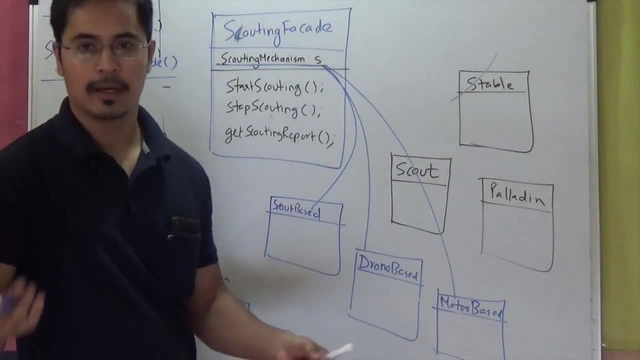 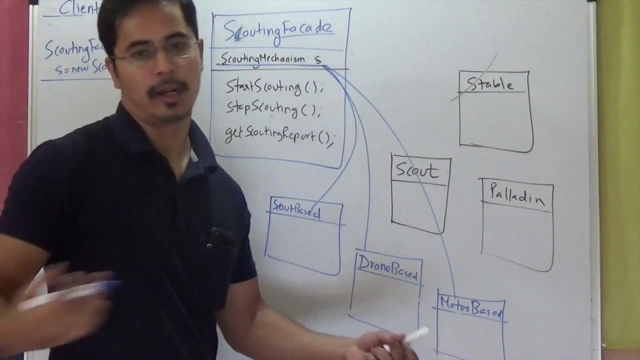 So that will be decided according to the era in which player is playing. So the constructor of the scouting facade code will initialize this S to one of these concrete implementations, But client doesn't have to bother about it. Client just has to create a scouting facade object. 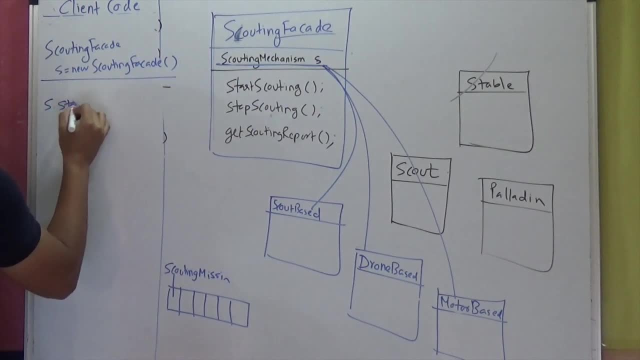 And say, S dot, start scouting. If this is your screen, right where you, this is where you are situated, you can just click on the mouse that in this direction you want to scout. So better, let's say, call it as direction. 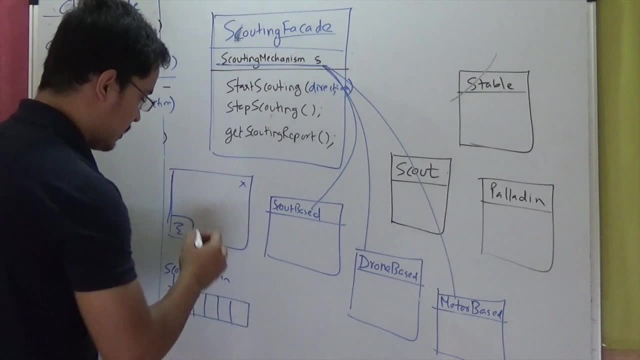 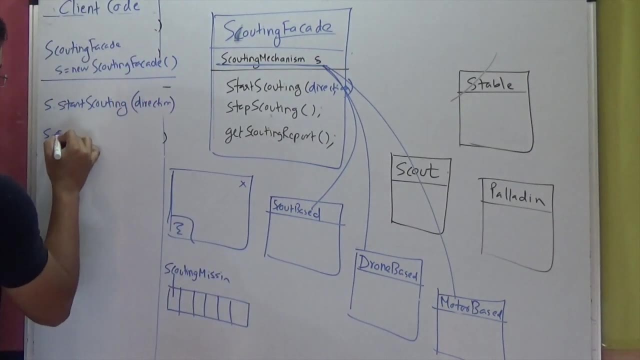 So you just have to specify the direction in which you want to scout, So you just have to click on that direction and it will start scouting. And at any point of time you feel like you can say S dot generate report. 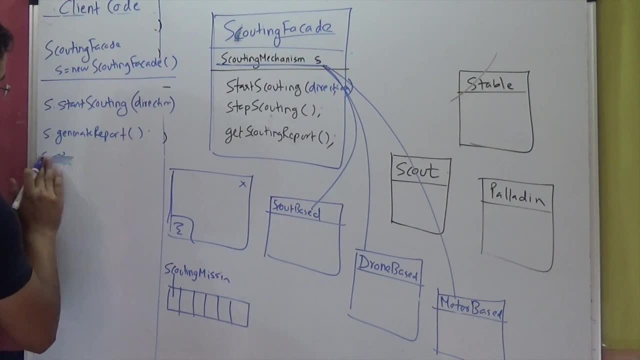 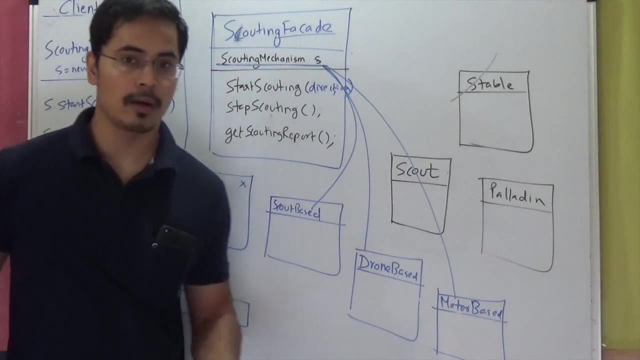 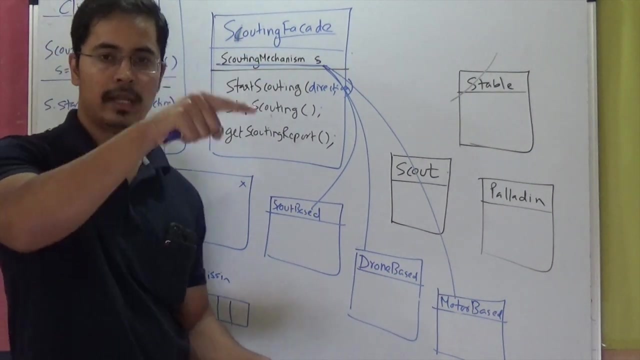 And you can also say S dot stop. And you can also say S dot stop scouting. if you want to stop scouting, right. So this is it. This is all you got to do As a player. you don't have to worry about creating a scout, creating a paladin, pointing them to next, next, next locations, so that they can eventually reach the enemy territory. 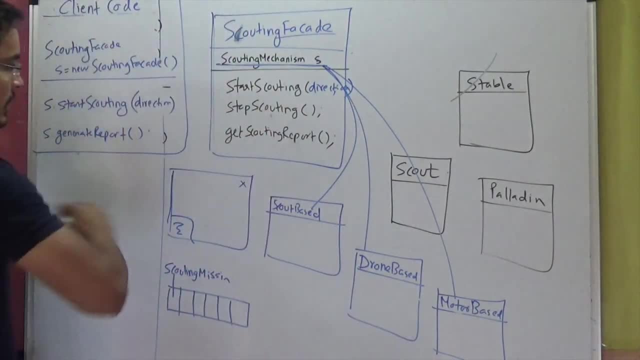 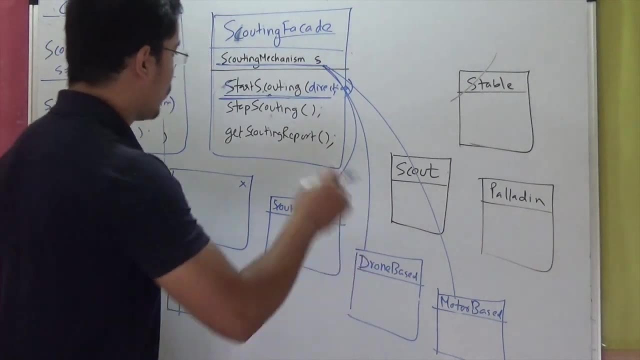 You don't have to worry about that at all, That all those activities will be taken care by the code that we are going to write in this start scouting method. Now let's look. Let's look at the code of start scouting method. right, 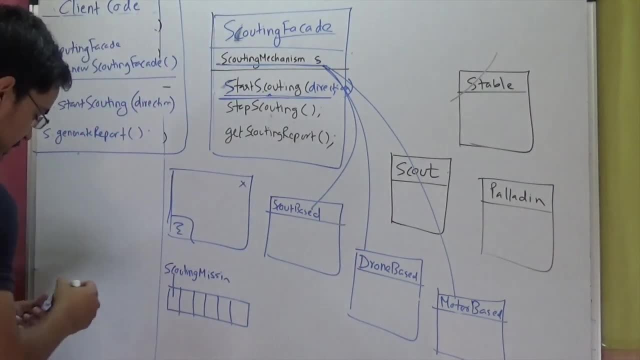 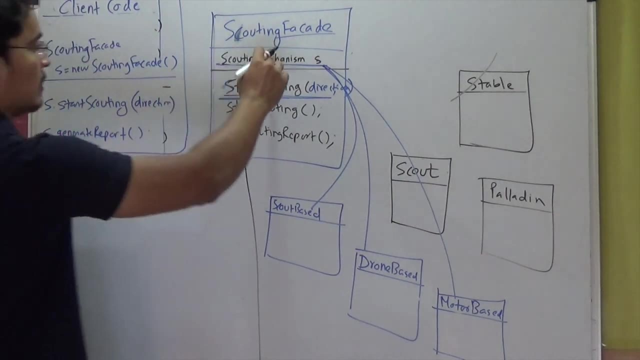 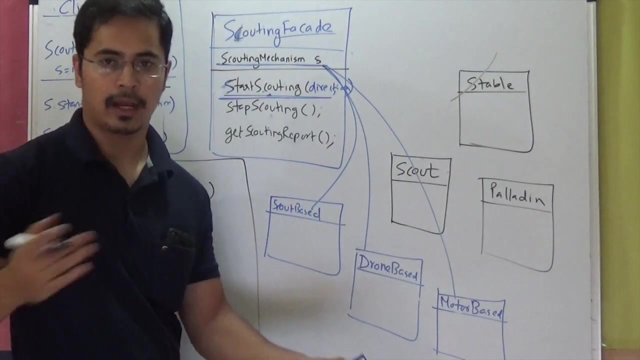 That we are going to call right From client, So I'll write it here. It has a direction right As a parameter. Now this facade class has a composed scouting mechanism. object Who will be initialized to one of the concrete mechanisms based on the era of the player right. 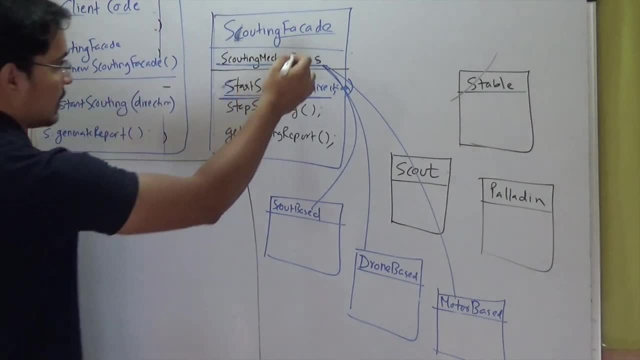 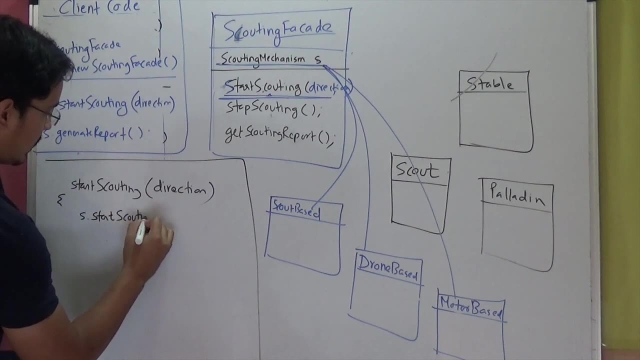 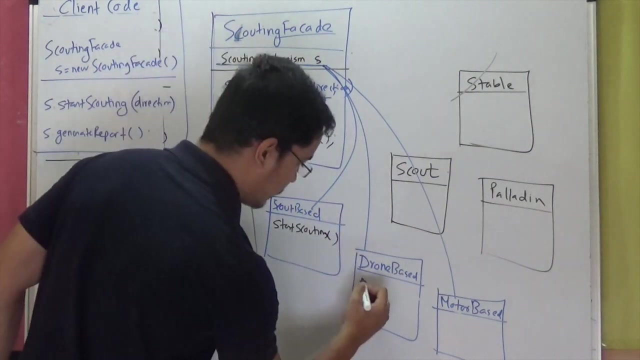 So once you have that initialization done right In the constructor of this, we can just say S dot Start scouting. So there will be start scouting method in each of this concrete implementations, right. So let's take an example of this, like horse based scouting, right. 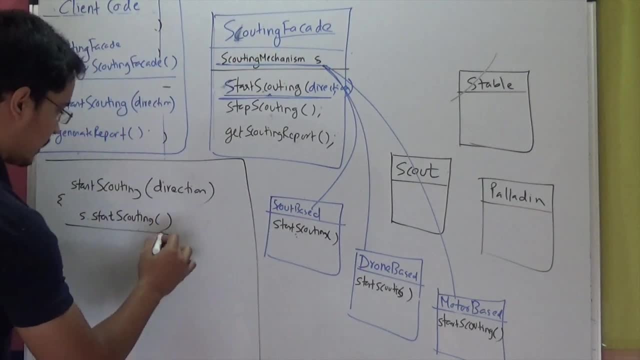 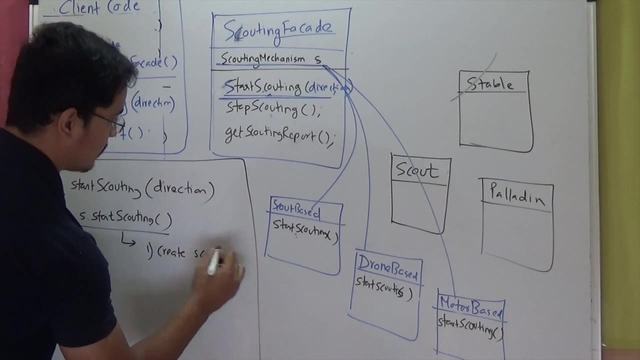 So this method, basically, which will be called here, will be something like this: So it will create first a scout, right? So it will create this entry, Right, So it will create this entry. Then it will create a paladin, right. 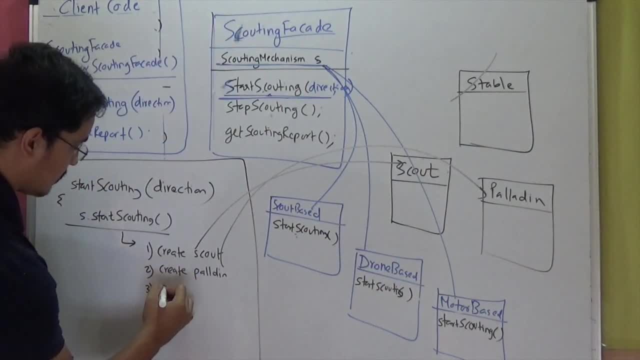 So it will create this entity for you. Then, whatever scout, let's say, this object is S and this is P, So S dot start exploring right, And it will use the direction. Then it will say: P dot follow right. 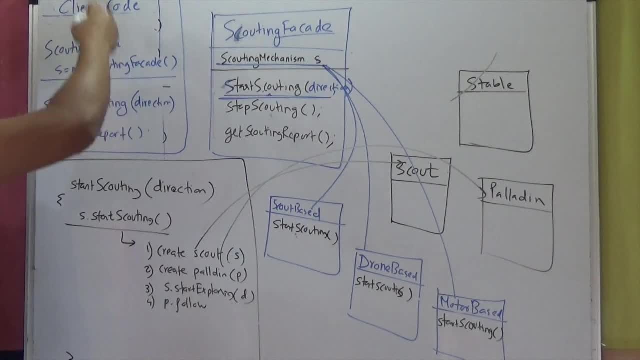 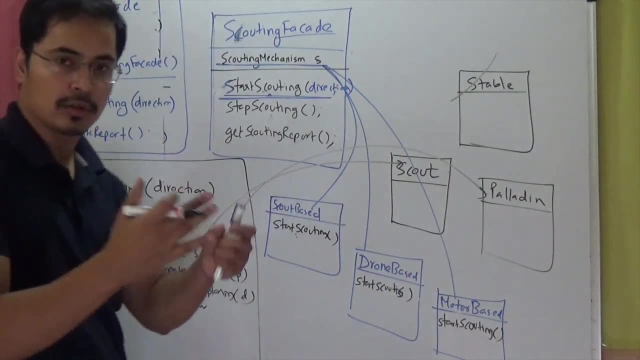 So all that code which we were earlier writing in the client side, that player had to do manually. Now we are putting, Let's say this, scouting mechanisms, So we are hiding those implementation details from the end client. That's what we are doing. 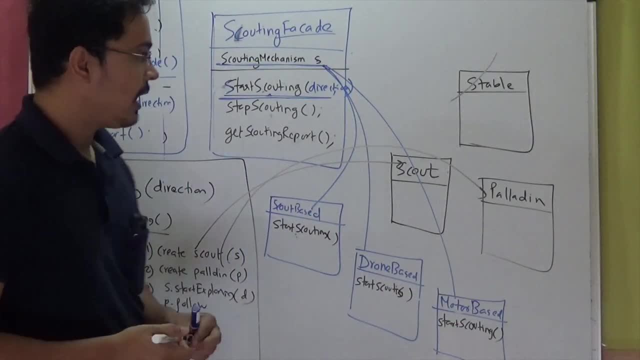 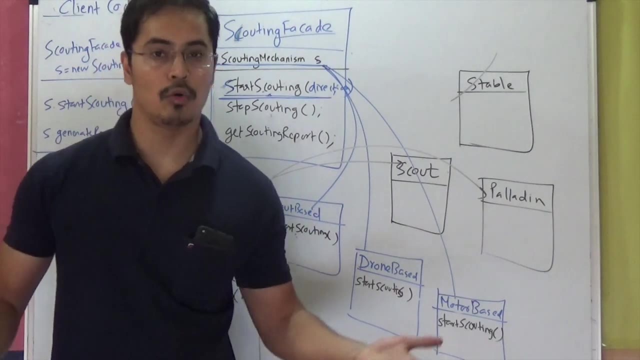 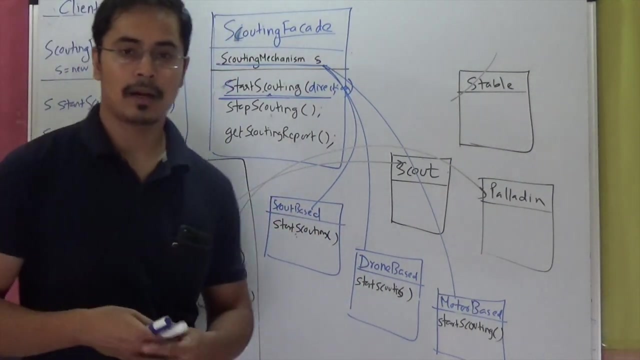 We are making it simpler for the end client right. What are the advantages of doing that right? What are the advantages? First, a facade can add its own smart code. It can add the additional functionality to the existing earlier code. For example, you remember I said there might be a river right. 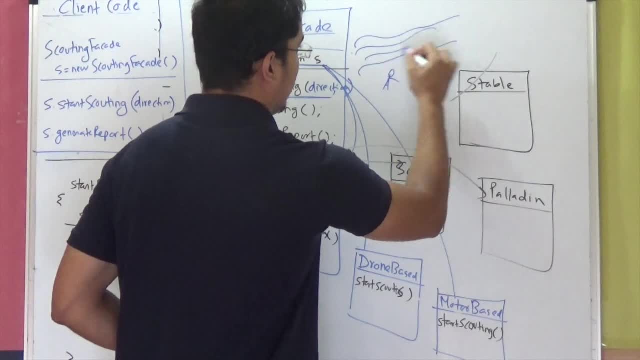 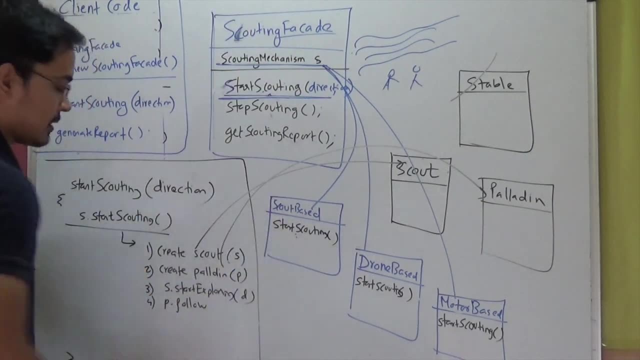 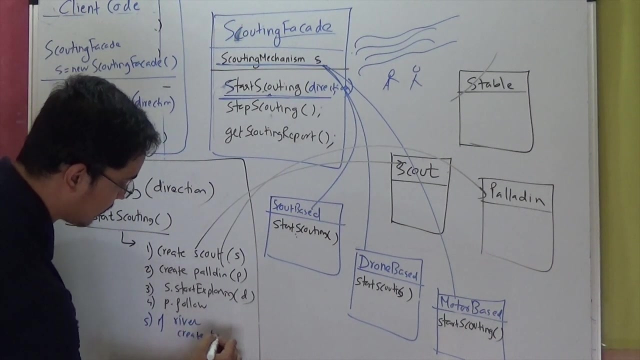 While you are scouting You might come across a river right And you can't cross it because only you have got horses. So here our scouting mechanisms can anticipate that. So let's say: if river create a boat, So they can create a boat for you, right? 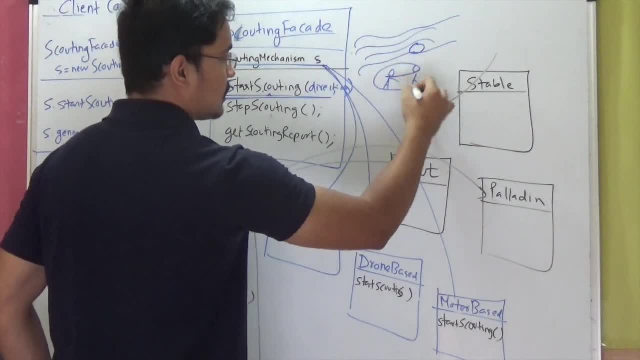 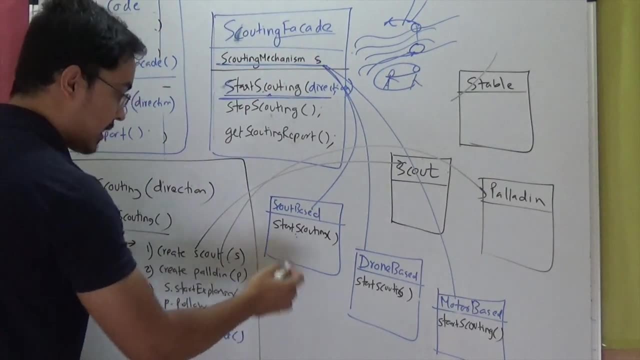 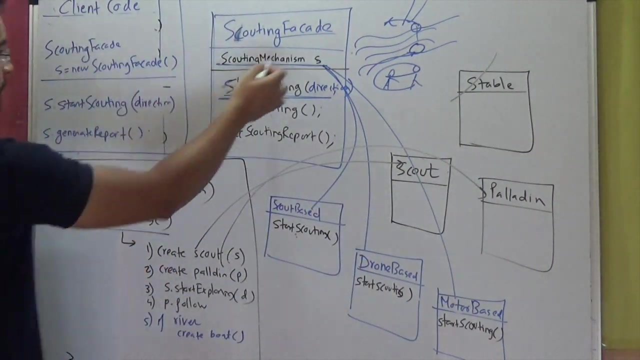 The boat will sail here. This two will get in that boat, sail here, get out of the boat and continue scouting. That code we can write Here right. User doesn't even have to know. All user is doing is that: create a facade object. 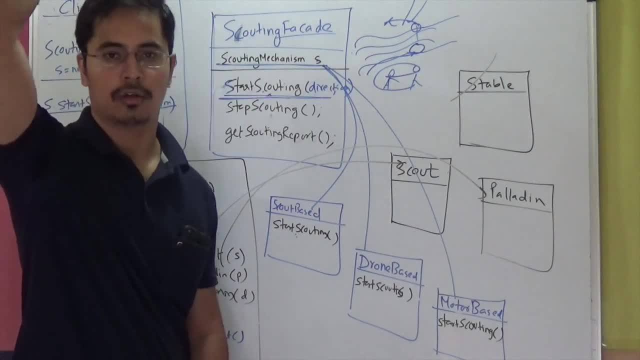 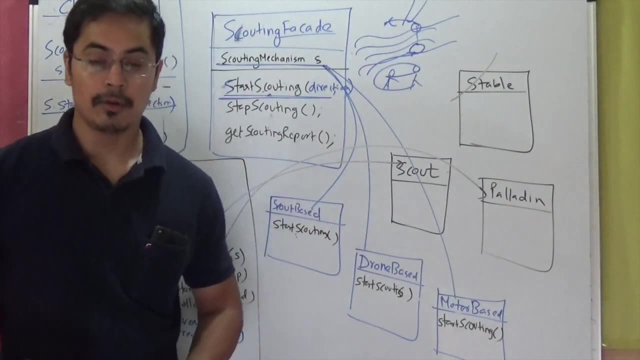 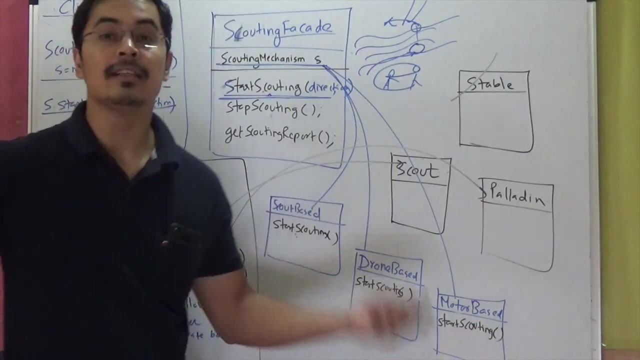 Say: start scouting and say west, east or north or northeast, northwest, That's it. All the obstacles in the scouting will be anticipated, will be taken care for in your scouting mechanism. codes right. User doesn't even have to bother about the scouting mechanism. 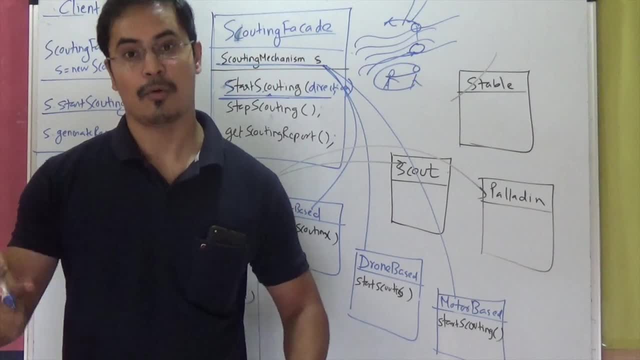 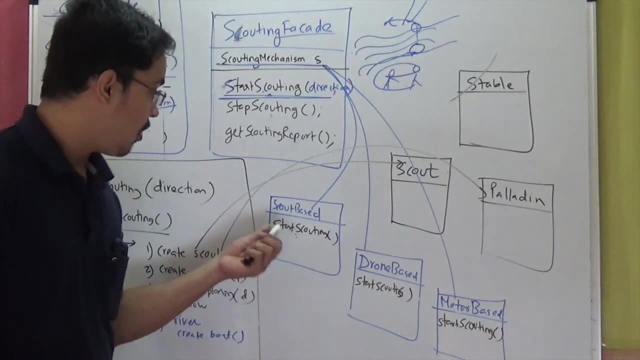 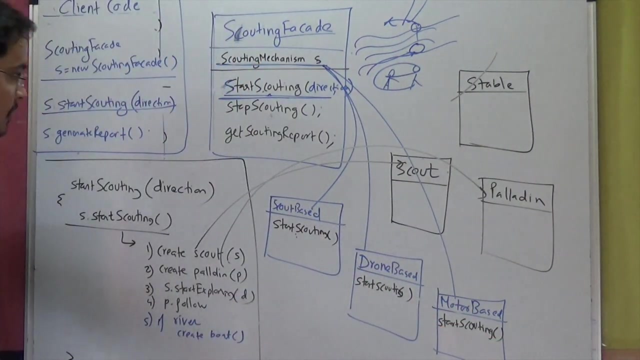 We can choose drone if user is in the ultra modern era. We can choose motor-based or tank-based if he or she is playing in modern era, or we can use the old style, horse-based, if the user currently is in medieval age. right, So all these details are hidden and we can add so much code. 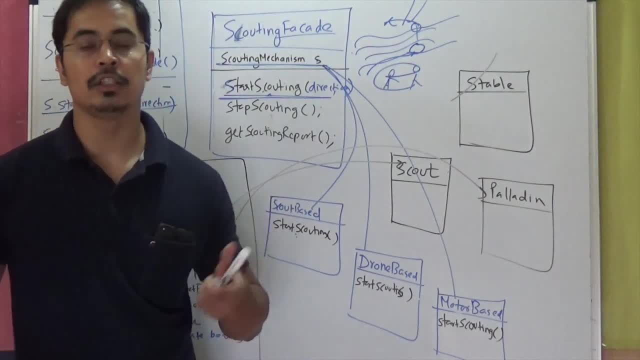 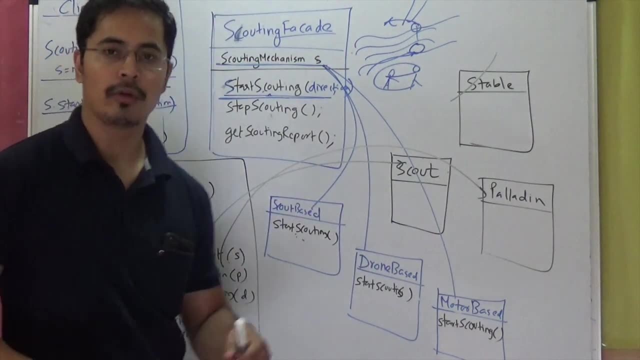 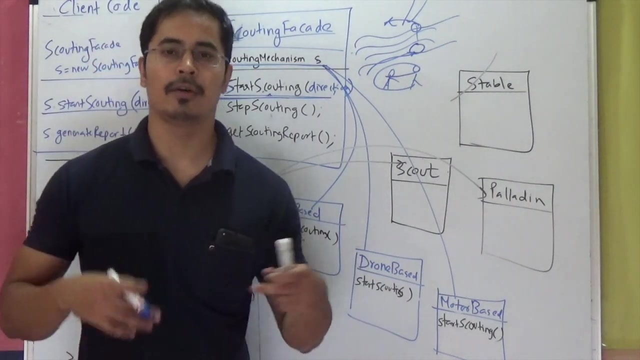 We can take care of all these situations. Let's say, scout gets killed, Paladin also gets killed. So this is our scouting code- will automatically generate new, Another scout, another paladin- and restart the scouting process. But this we are talking about functional terms. 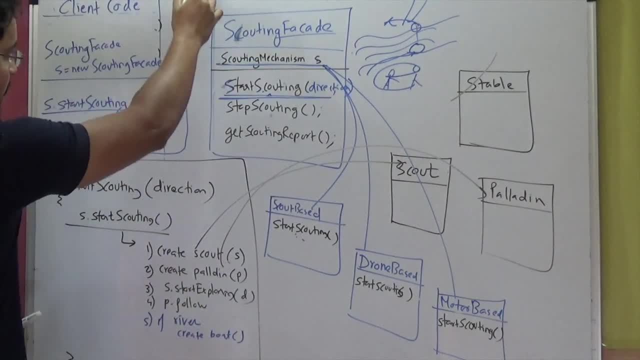 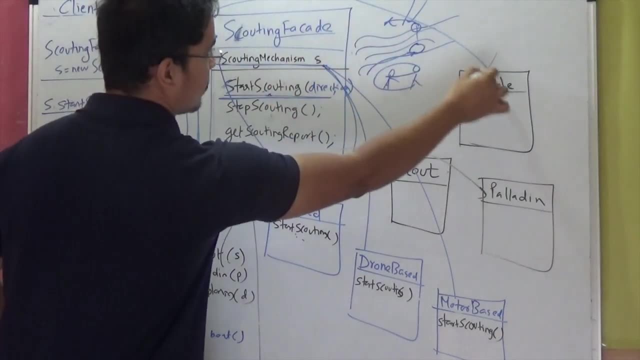 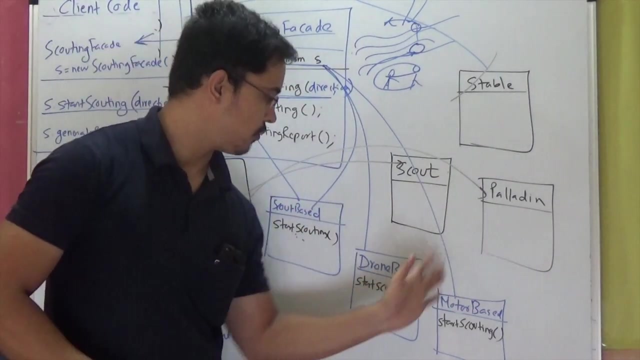 The most important thing that you can see is we are decoupling. We are decoupling the client code from the actual implementation. right, This is the actual implementation. all this, We are decoupling the client from it. The advantage is that we can change this code tomorrow. 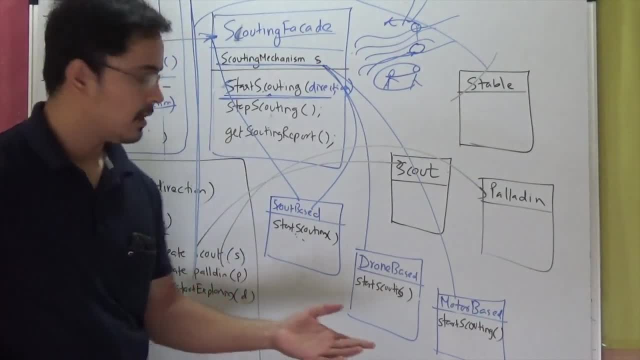 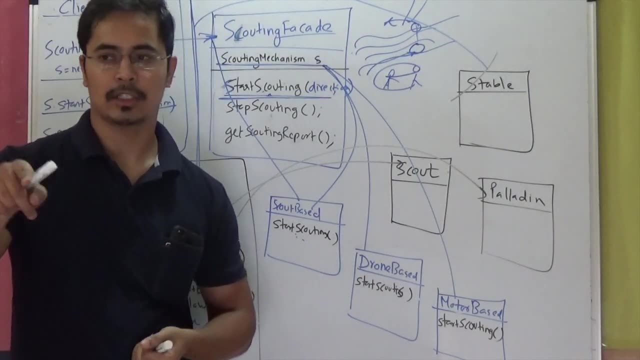 We can change the behavior of this scouting mechanisms And client doesn't have to know. The client code doesn't have to change, It remains the same. It has to just start the scouting mission, stop the scouting mission and get the report. Meanwhile we can change a lot of code here. 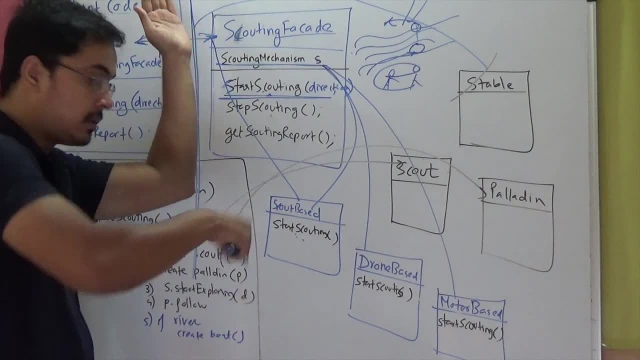 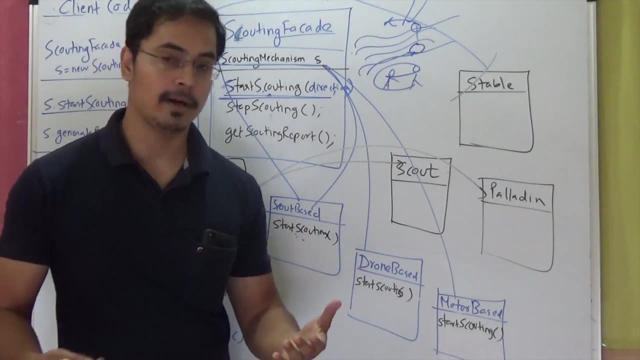 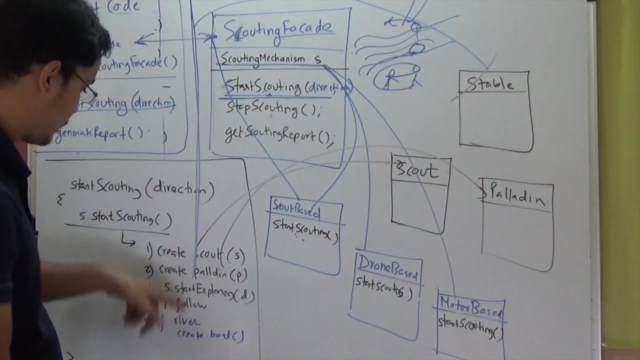 We can add some new possibilities- what if this, what if that, what if this, what if that- to the code. But it is loosely coupled So we don't have to change the client code. So facade pattern says that for your complex subsystem right which you are currently using through invoking methods and object creation in a client code, 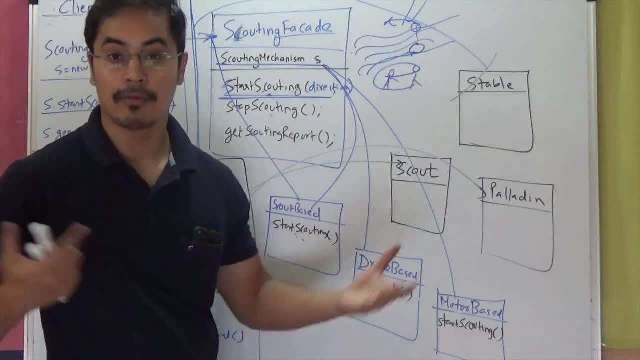 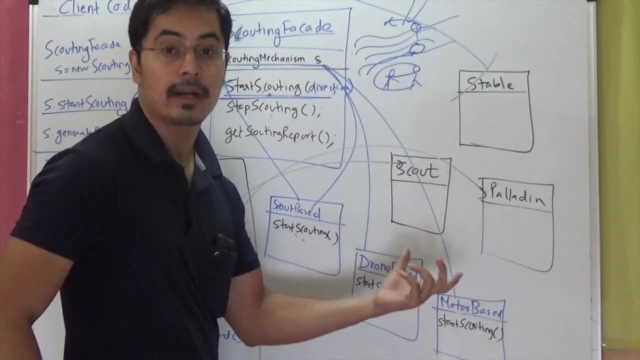 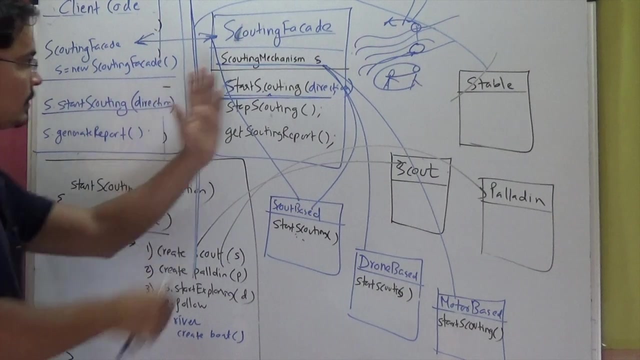 Create a simplified interface. create a simplified interface for that complex subsystem and give access to the functionality of that complex intended functionality of that complex subsystem to your client through easy to use interface, easy to use methods. This is your facade pattern. One more advantage: 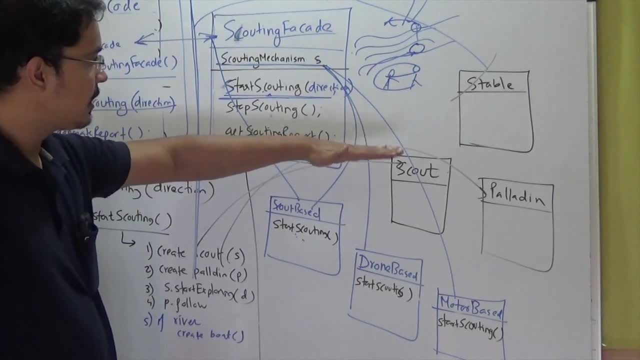 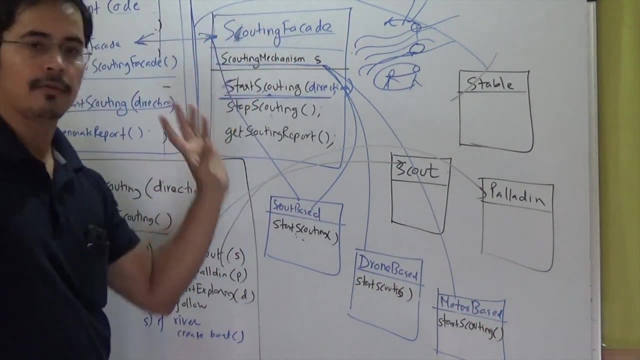 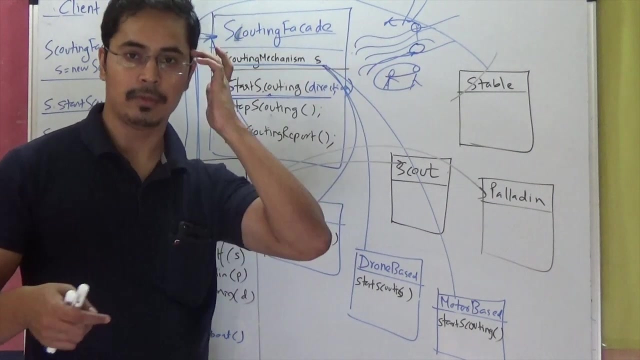 The way facade works is it doesn't completely hide the participating entities from the end client Right. So despite using facade, the client, that is, the player, can still create an individual scout Apart from this facade mission. he can still choose to go for individual scout. 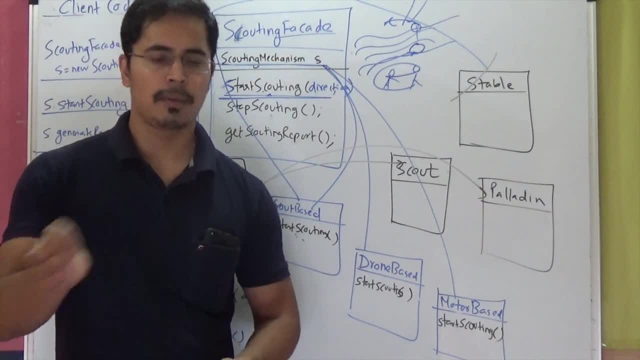 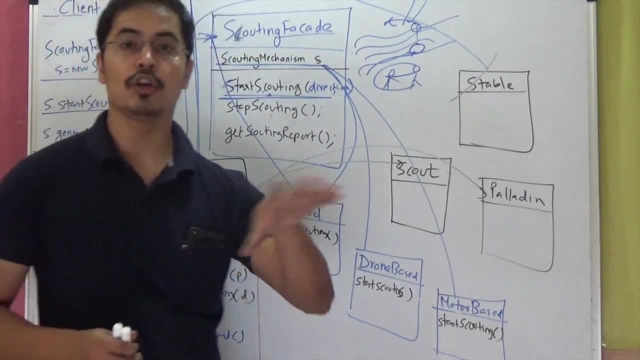 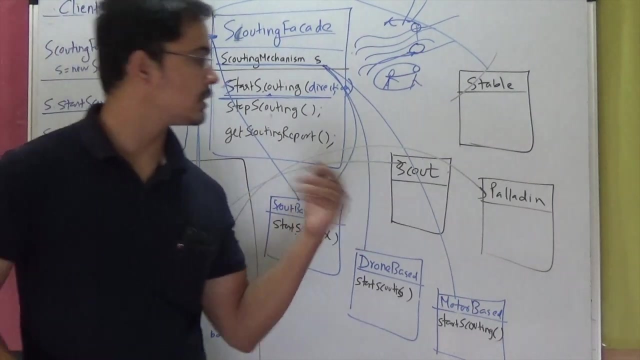 Let's say, for some other purpose, for keeping a watch on his own territory. He can still create a paladin, So he can still access the individual components of the subsystem for which facade was created. So it's not like, now that you have a facade, you can't generate your own facade. 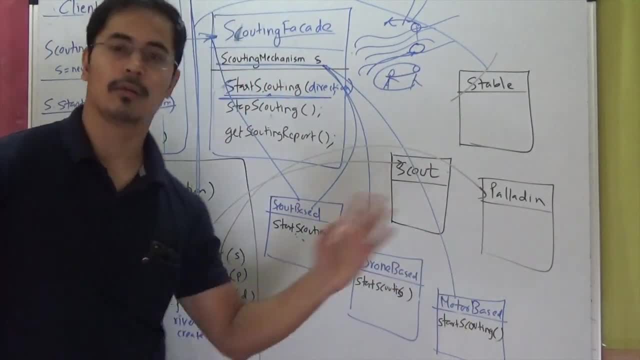 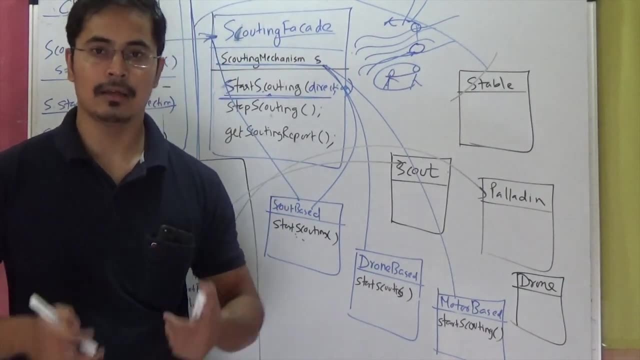 Or you can't generate paladin or stable or any of this or drone. Let's say we have a drone class, You can still have your own drone. That is one more advantage with facade: It doesn't restrict you from accessing the individual components of the subsystem for which the facade was created. 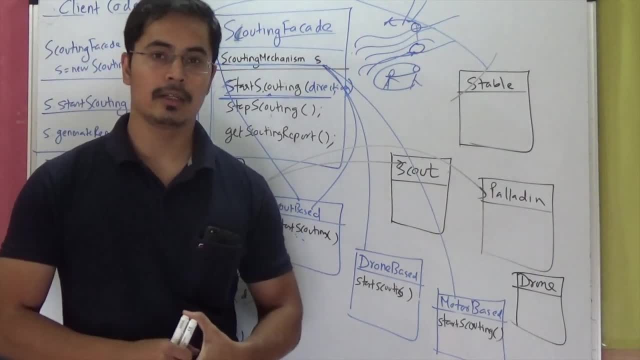 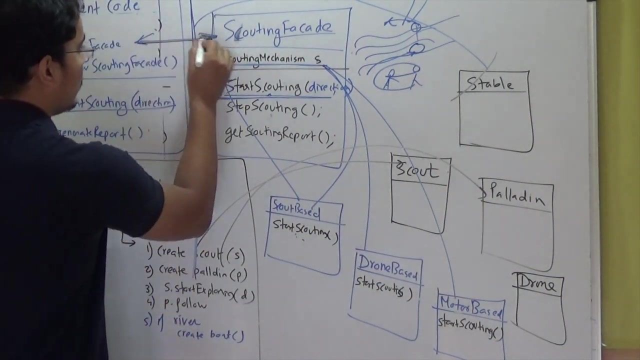 Eventually facade follows the object oriented design. principle of least knowledge. So what is least knowledge principle? Least knowledge principle says you should only talk to your immediate facade. So here this client code object is only talking to an initial or immediate friend object.